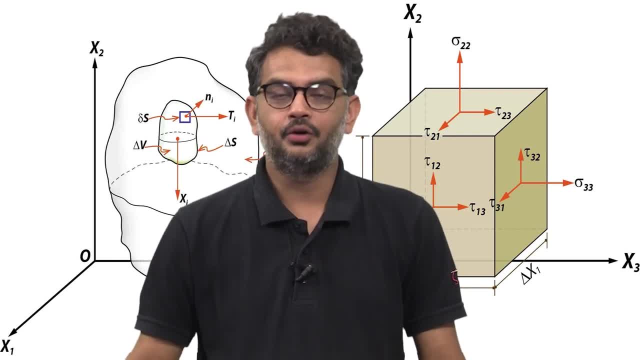 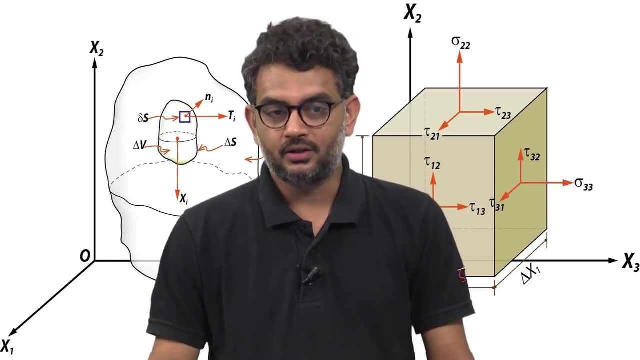 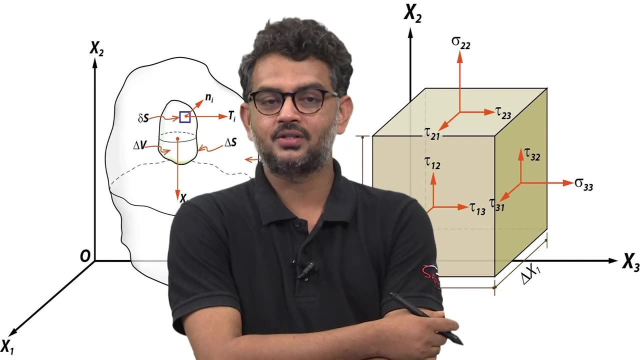 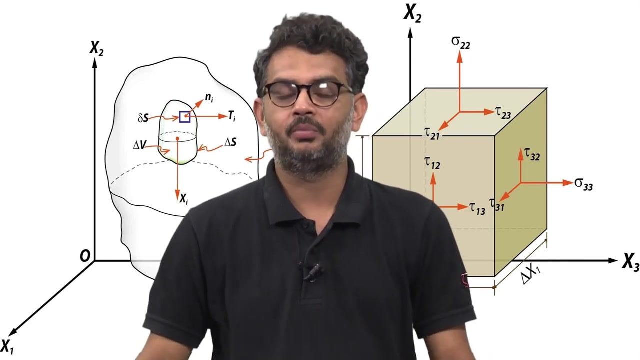 subject. Today we will cover a new topic very much related to the topics we covered before, strain, and this lecture will cover stress, and I must say that in structural geology, stress is one of the very important components or pillars. without understanding of this particular topic- stress- 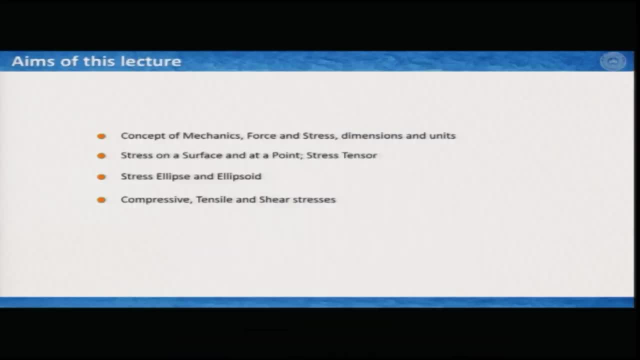 In the structures that we see in the field. subject: stress includes a concept of mechanics, of forces and stress, their dimensions, their units. Then we will slowly move to some sort of very basic mathematical operations to understand what is the stress on a surface, what is the 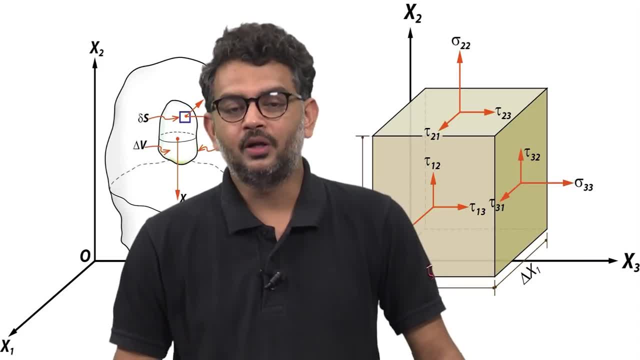 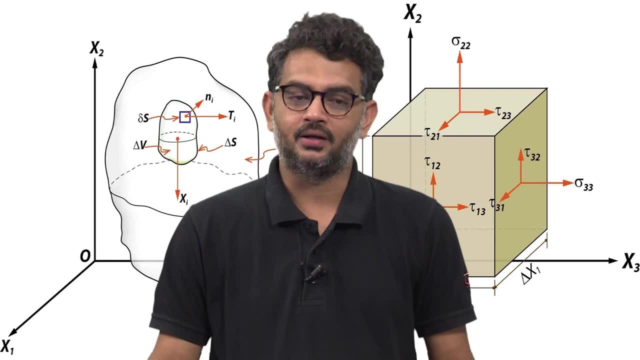 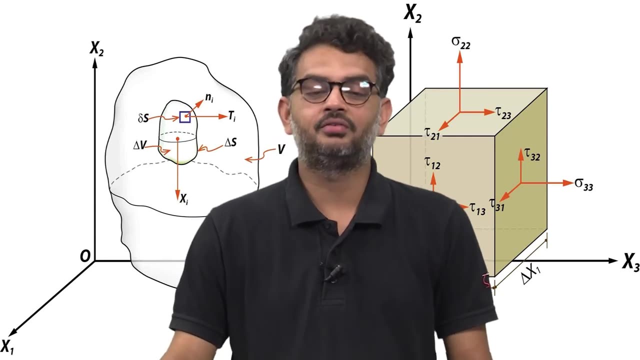 stress at a point, and then we slowly move to a concept that is called stress tensor. After that we will look at stress ellipse and stress ellipsoids, and we will conclude this lecture with the concept of compressive, tensile and shear stresses. We will also look at what 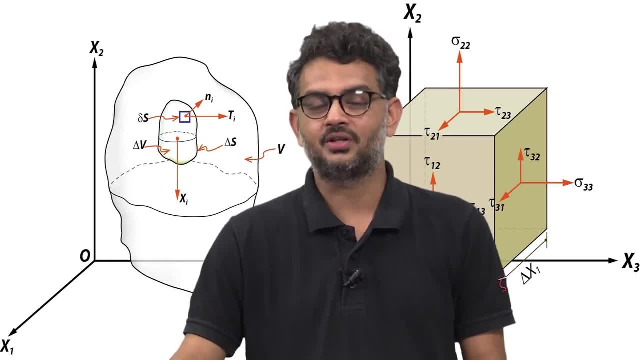 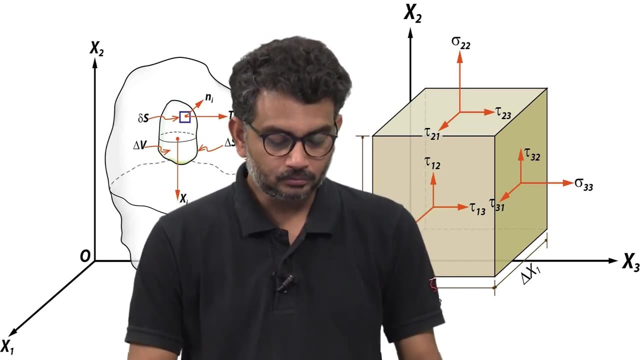 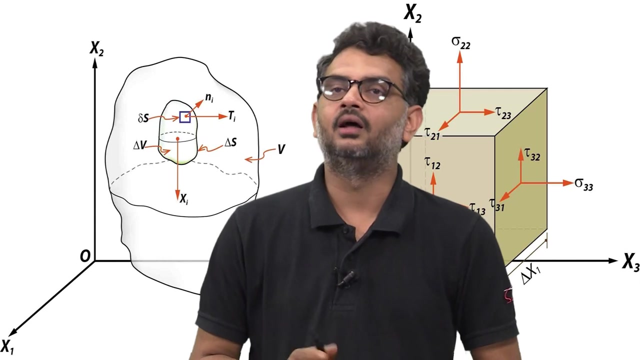 are positive stresses and what are negative stresses that we consider in particularly structural geology, and how do these concepts that we particularly apply in structural geology do vary from other structures? Now, it is very important to feel that stress is something that we do not see, but we feel. 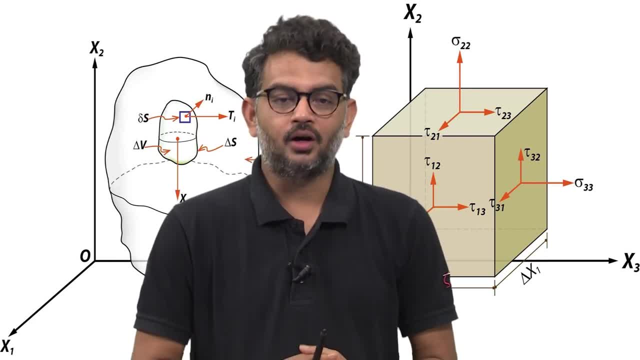 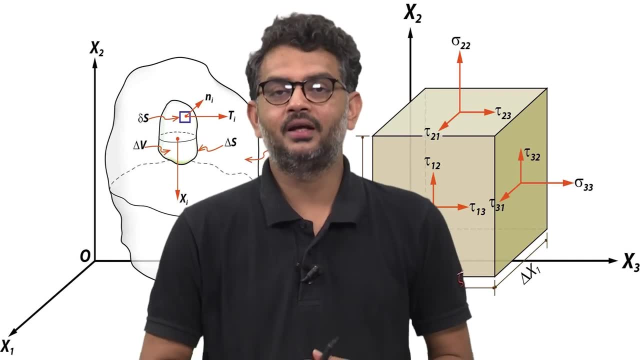 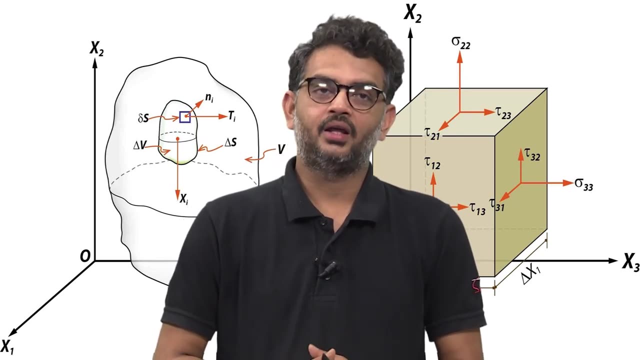 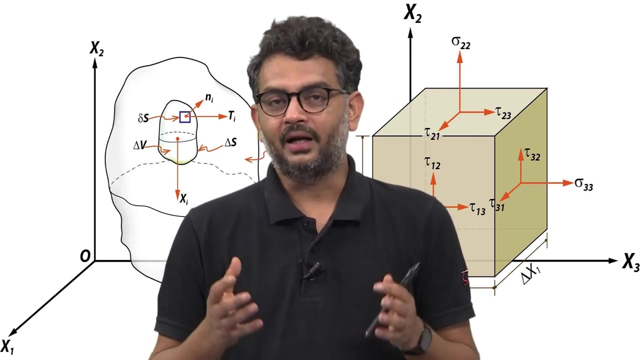 its effect In the context of geology or, to be very specific, structural geology. we are convinced now, so far the lectures we have, that rocks do get stressed And if you have strain in your rock that you are considering with, that means it must. 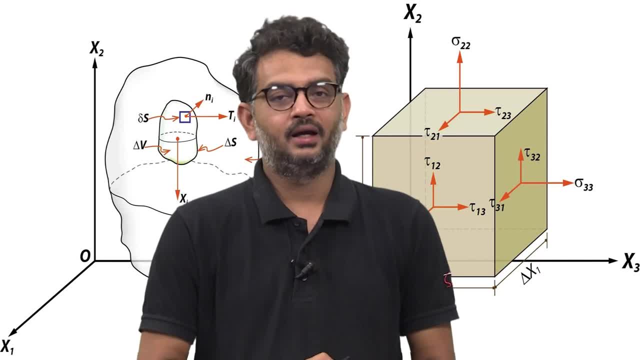 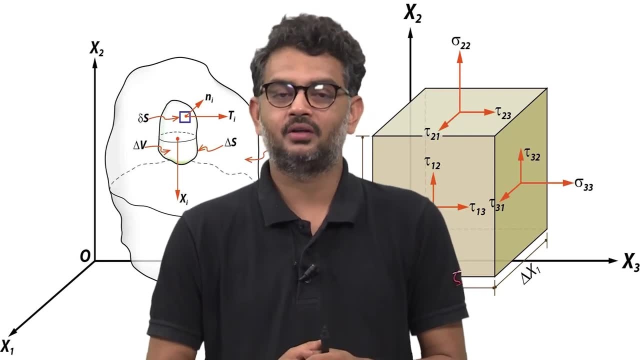 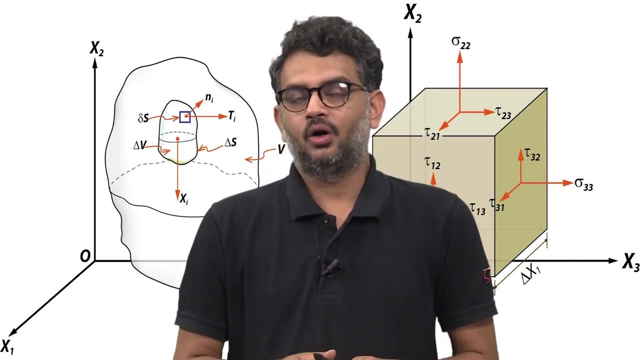 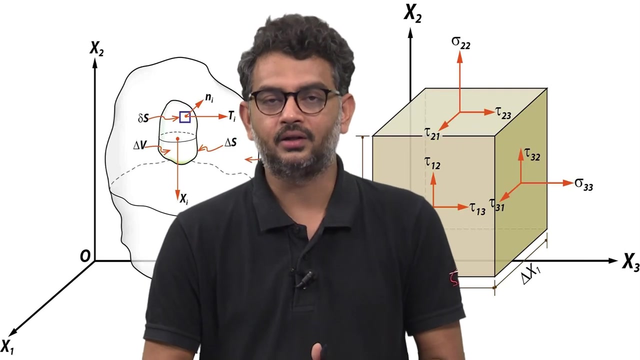 have moved from its original place and at the same time it also has changed its shape and dimensions. that means it got distorted. Now to achieve this strain in these rock masses, who does it or who is the driving mechanism responsible for this strain in the rock? And the answer? 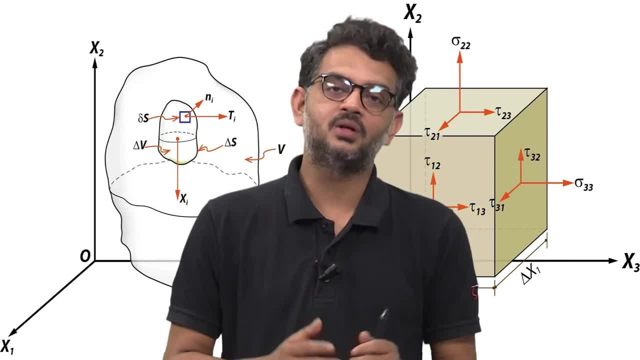 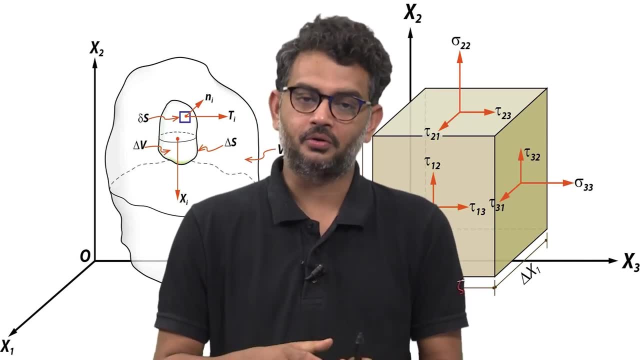 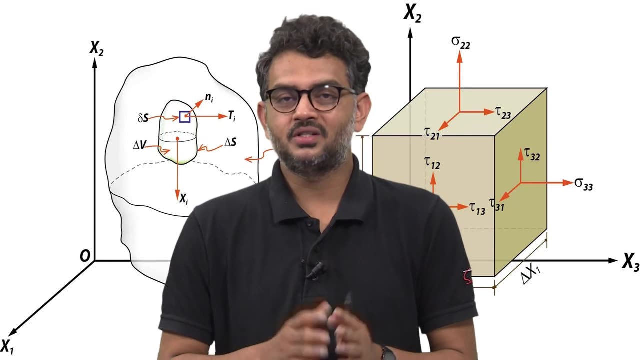 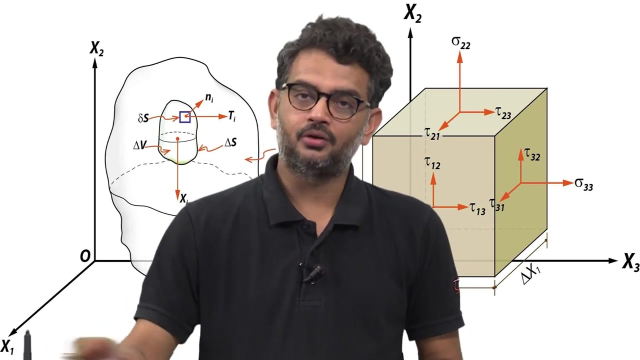 is that this strained material, when it was getting strained, it must have experienced some sort of natural forces or pressures or it was subjected to some sort of natural forces and pressures. And I repeat that we do not see these pressures or forces, but we feel it and this is what we would like to continue in these lectures. 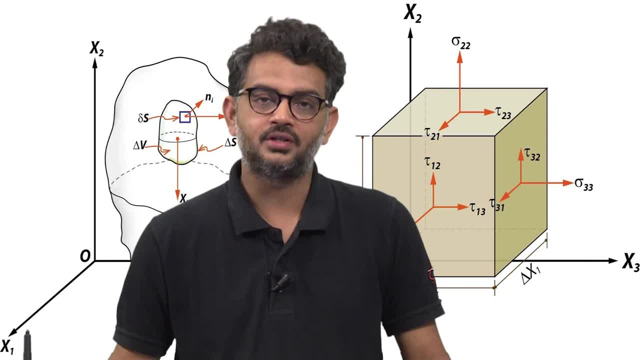 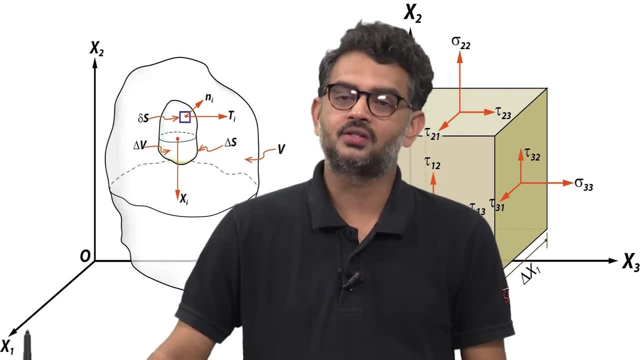 But before that, let us have some basic ideas of this general topic overall. Now, first of all, you must have heard this word stress from your school life. you must also have heard this word force again from your high school levels, And we know that the forces 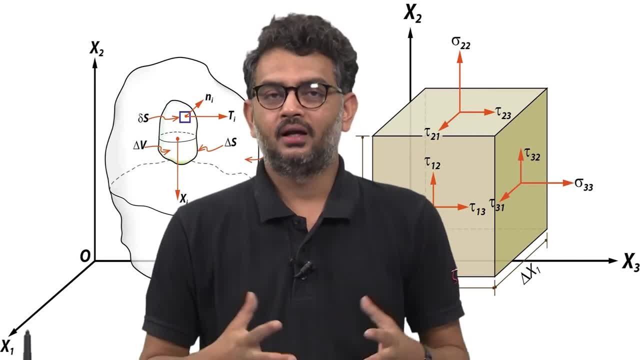 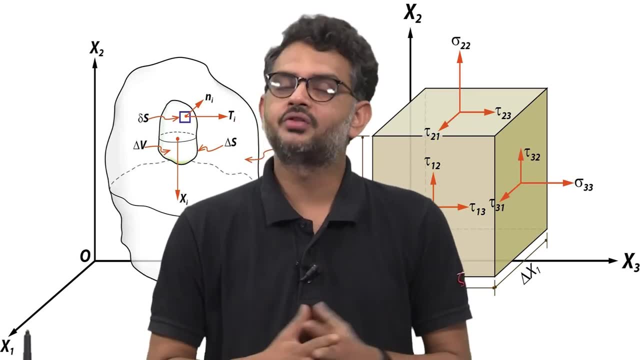 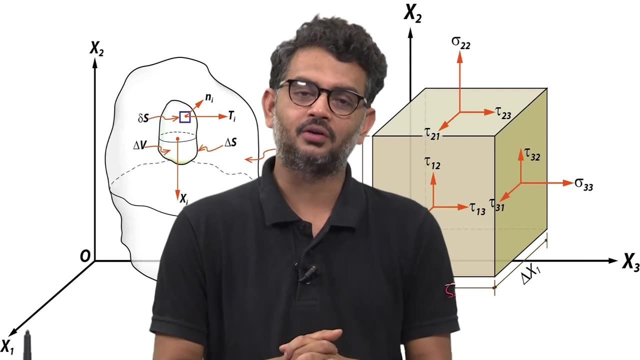 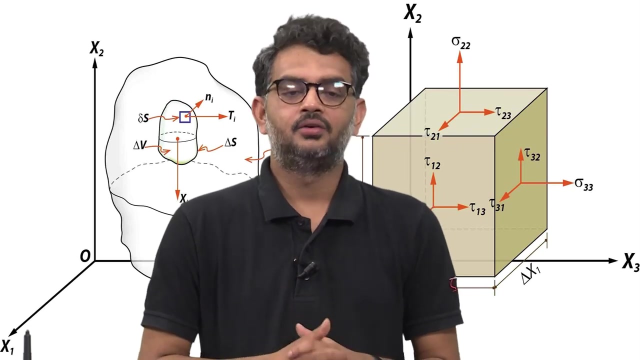 or stresses. whatever we consider these two things, they have to act on some materials. Now, rocks, as we can figure out, that is essentially some sort of materials, special kind of materials you can think of. But so the study of deformation of rocks under forces fall, certainly falls. 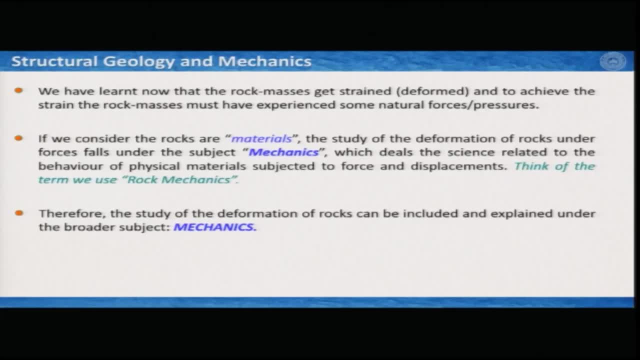 under the subject mechanics, And mechanics is something that is a topic, is sort of a topic that we cover in physics mostly. that deals the science related to the behaviour of physical materials. that means that you can visualise, you can feel, you can touch it subjected to force and displacements. 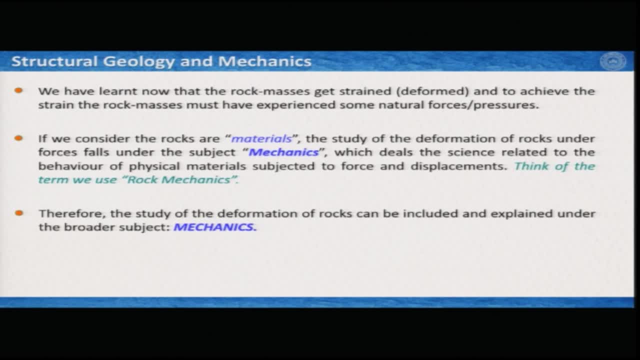 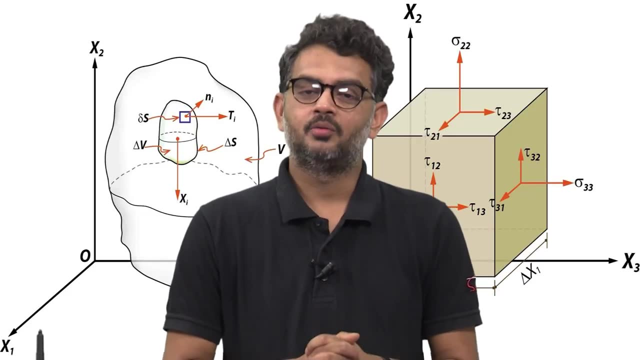 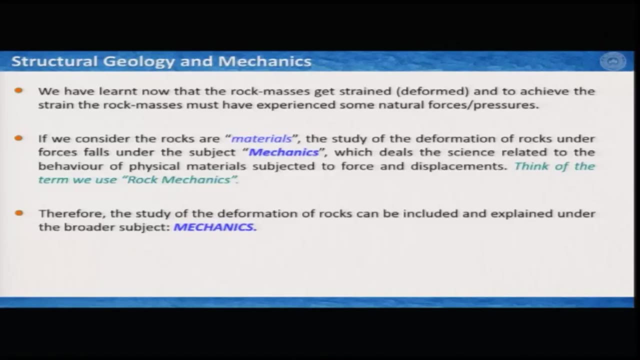 So, therefore, if we consider rocks as our materials, then we have learnt that these materials, rock materials, do get strained Because of some sort of forces and pressures. and if so, then we can study the effect of forces and pressures on the rock materials to achieve some sort of strain. we can study. 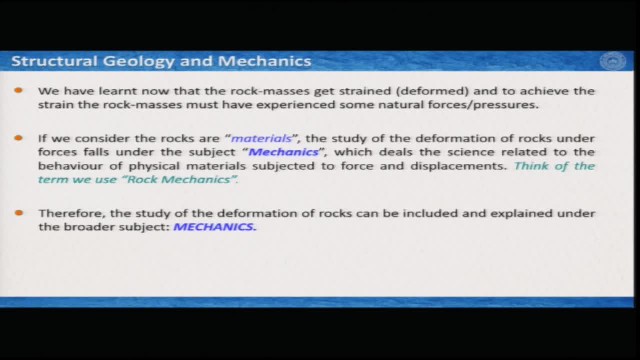 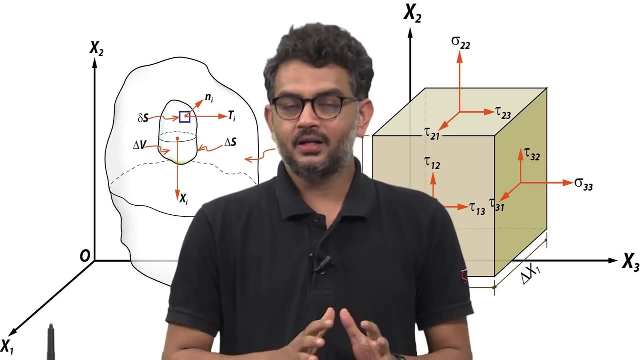 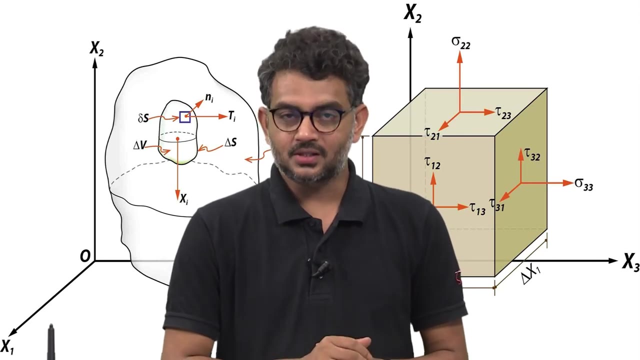 it under the broader umbrella of the subject mechanics, And we generally call it- I am sure you have heard this term- rock mechanics, So it is. it is very interesting that we will see how rocks as well like all other materials, we can study under this subject of mechanics And at the same time we will look at that. 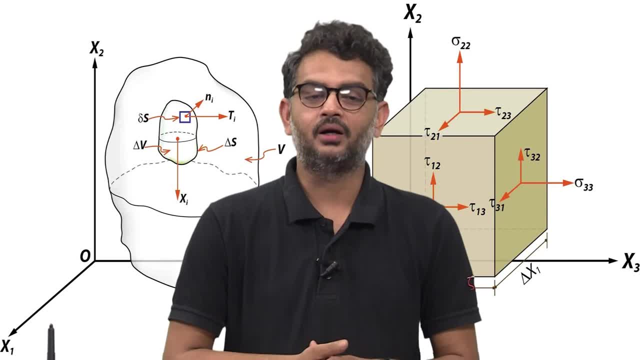 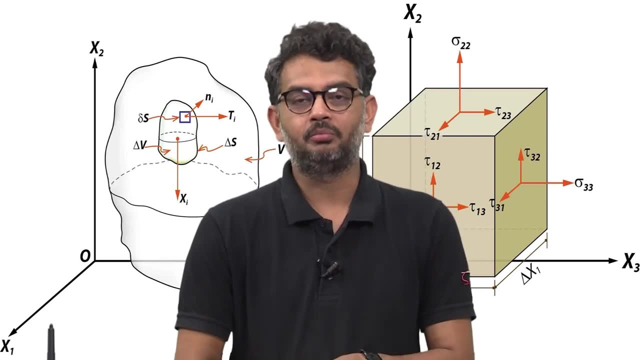 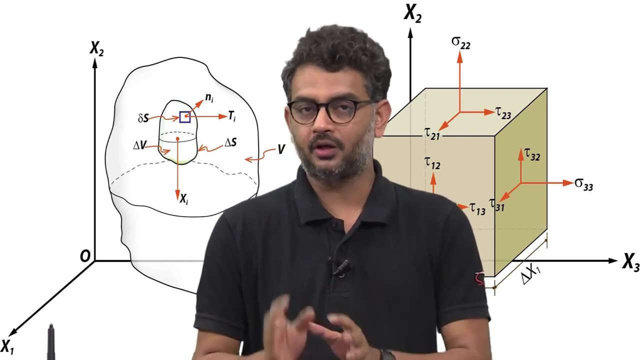 there are many branches of mechanics, So you must have had quantum mechanics, you must have had continuum mechanics. solid state physics is also a type of mechanics that people do study, And we will see that in rock deformation or in structural geology. we will consider a particular 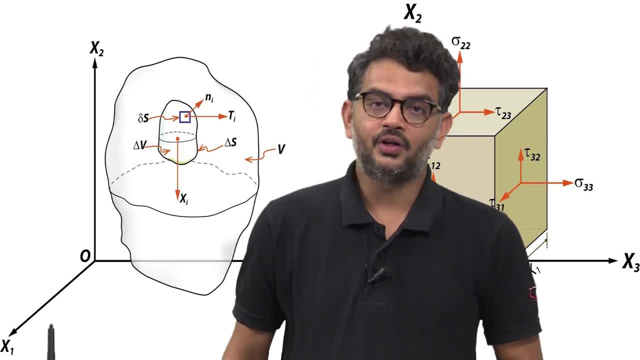 type of mechanics, and this is known as continuum mechanics. 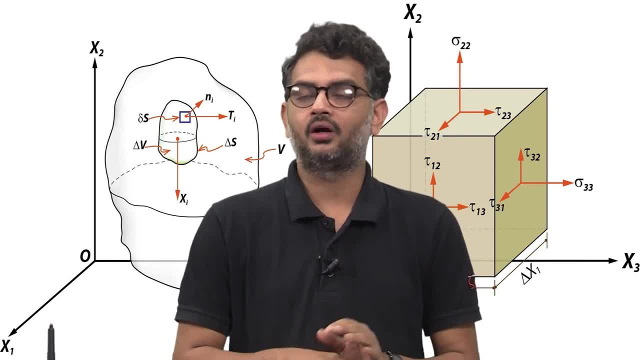 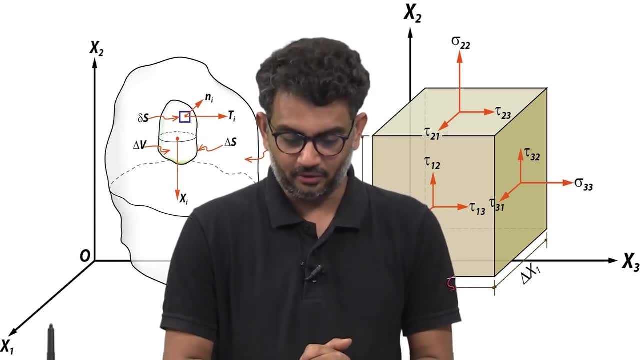 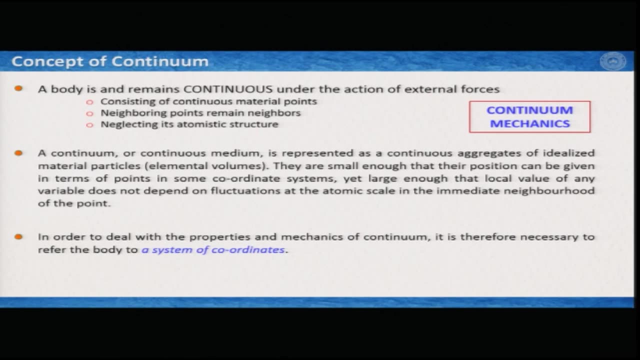 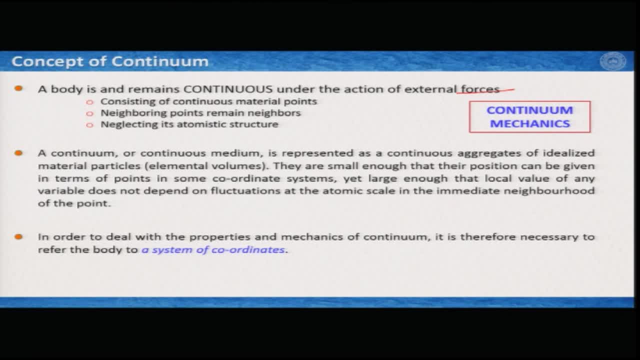 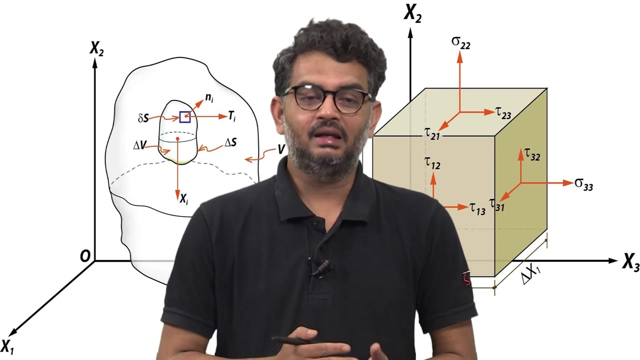 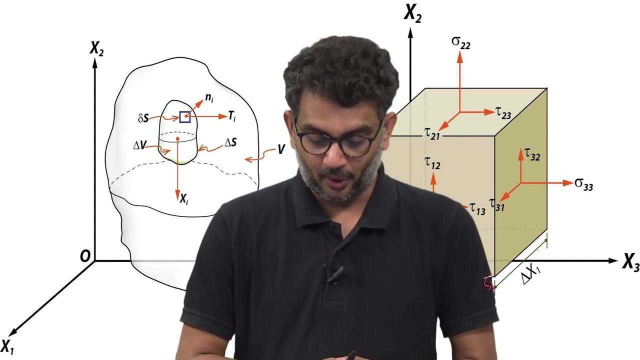 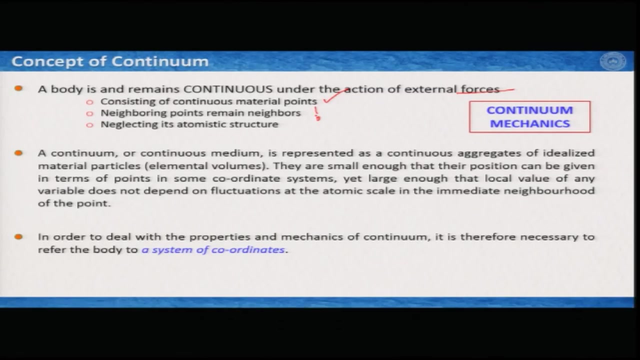 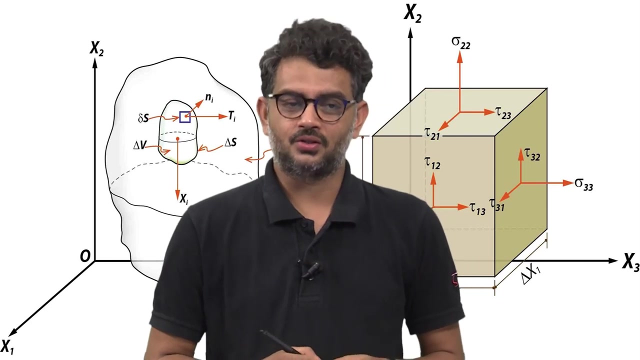 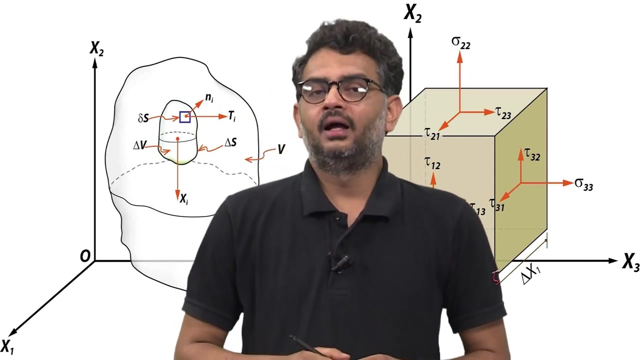 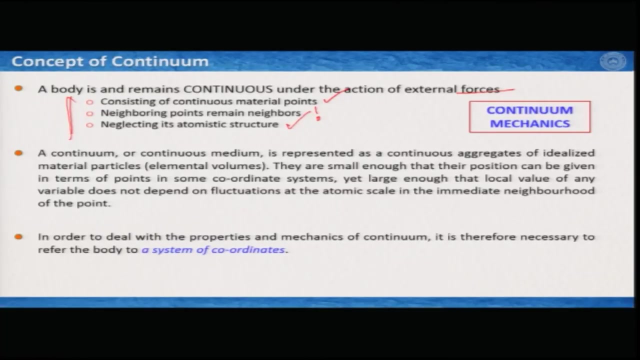 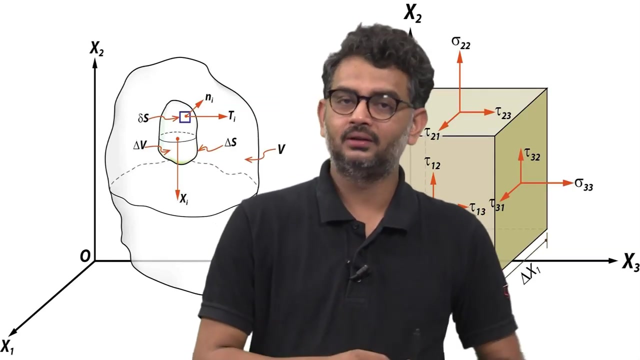 any variable does not depend on fluctuations at the atomic scale in the immediate neighborhood of the point. So this subject is being studied under a sweet spot that it is not that small. 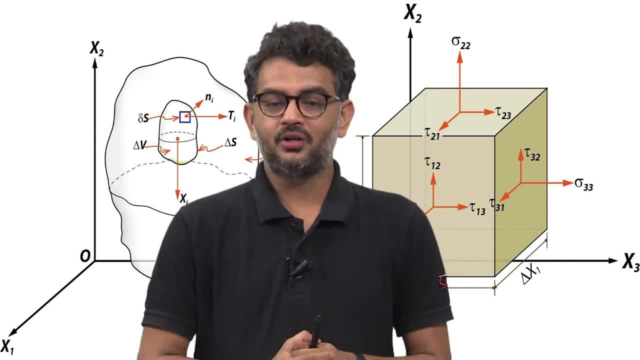 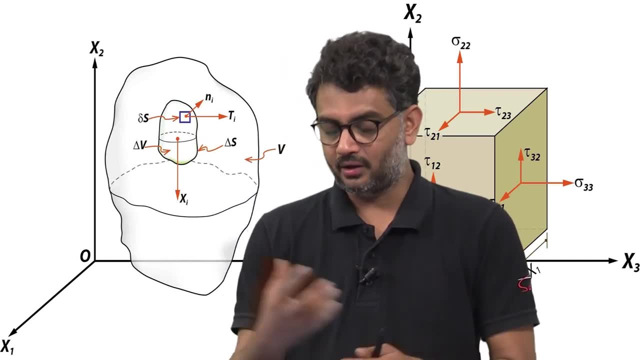 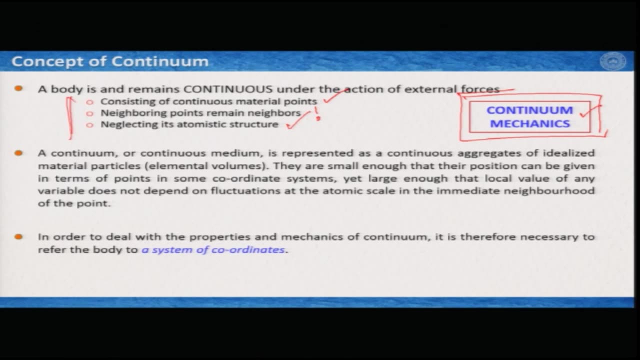 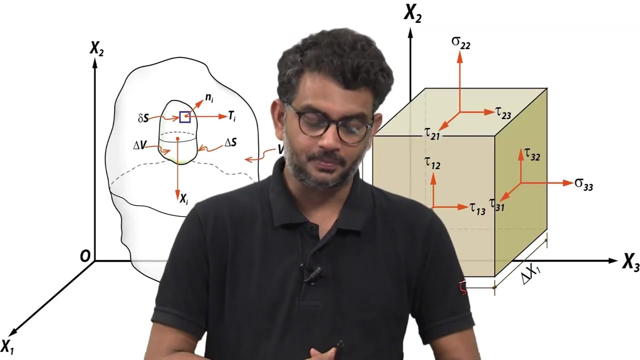 that you cannot plot it in a coordinate system. but at the same time it is not that big that some small fluctuations at the atomic scales can affect your system. Now again, this is little confusing for studying the earth, because earth is really big and a little fluctuation somewhere can cause large fluctuations in other places. So again there, 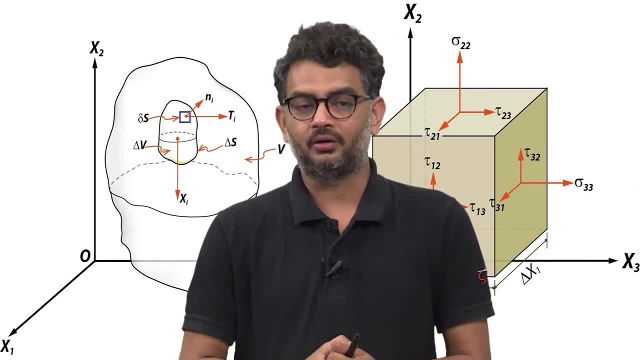 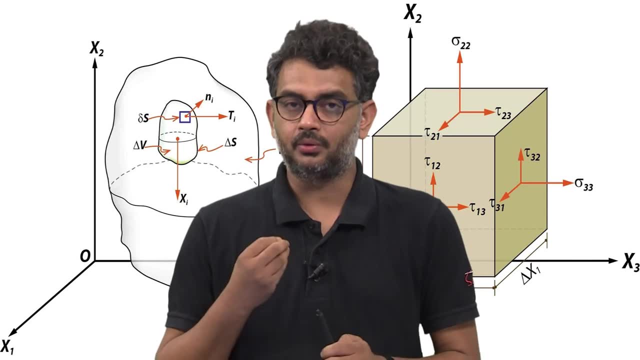 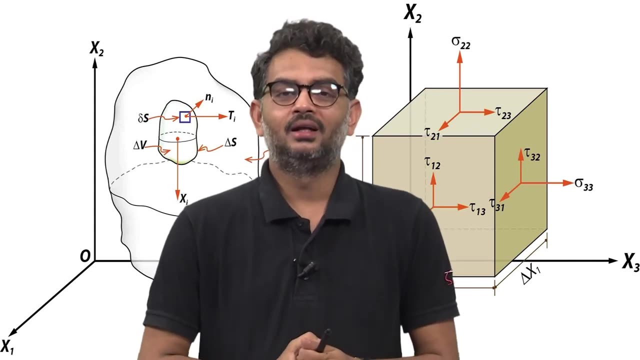 are some sort of approximations and, what is most important, that when you model something or in your study something, you actually ignore some very micro scale features. What I try to say here that if you are studying a grain or grain scale processes, then you do not take care probably what is happening at the top. 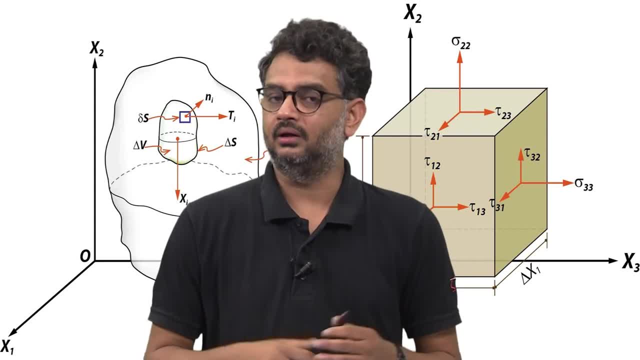 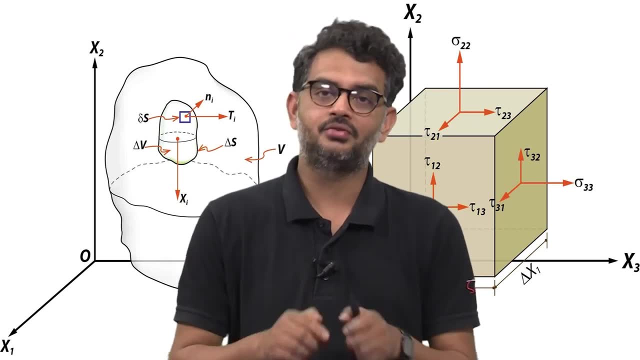 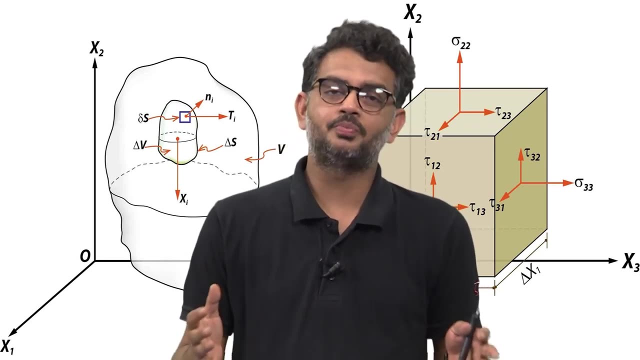 of the mountain, or you do not care if there is a lot of deglaciation or there is a huge rainfall. These things probably do not affect your scale of study. Now, if you go to little larger scales, for example if you are studying a rock specimen, then you do not take care. 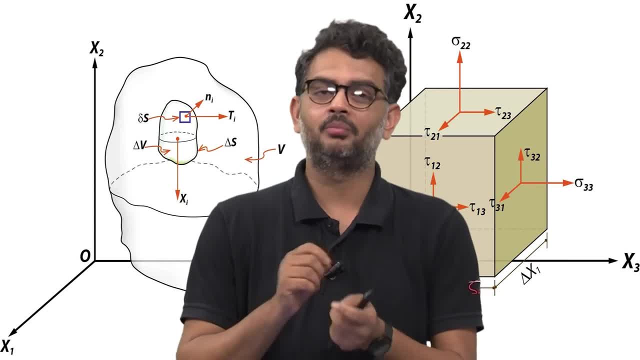 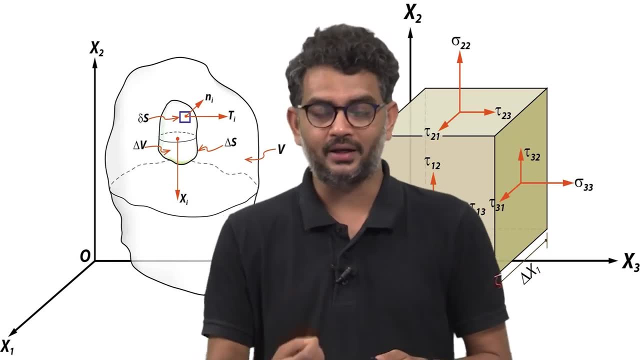 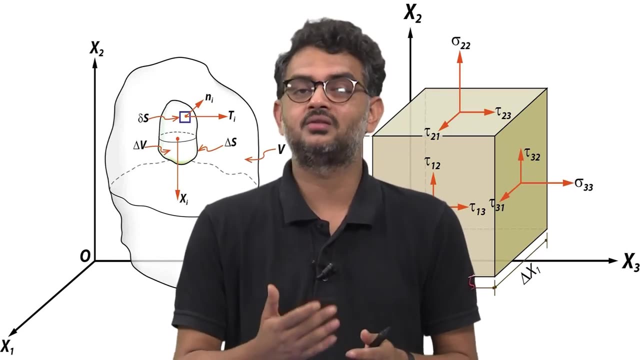 of these internal features inside a grain scale, For example, dislocations or some crystal vacancies or some interstitial impurities inside the crystals. When you study a rock specimen, you do not consider all these little things. you ignore them. You believe that these things do not affect this. If you are. 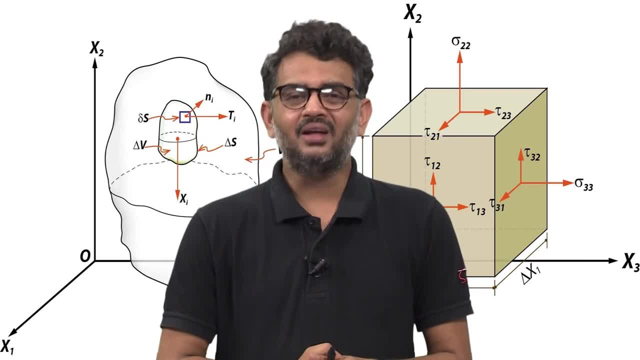 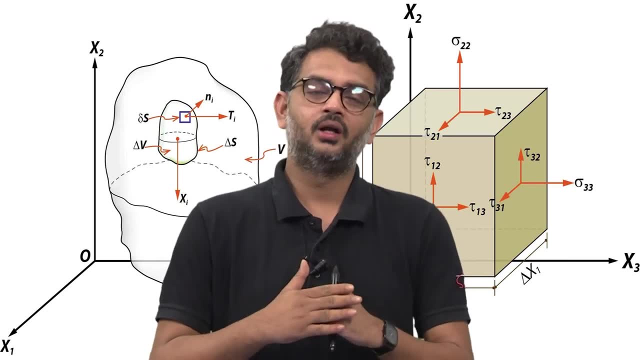 studying a scale of plate tectonics, then you do not consider the different layers that you see in rock systems. For example, you do not consider a shape of the rock, the shape shell layer or sandstone layers and then limestone layers and so on. These things we ignore when 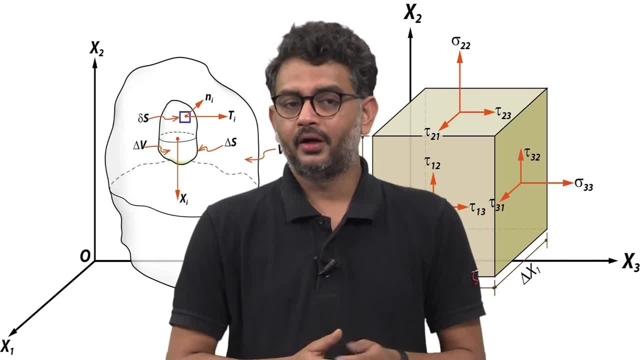 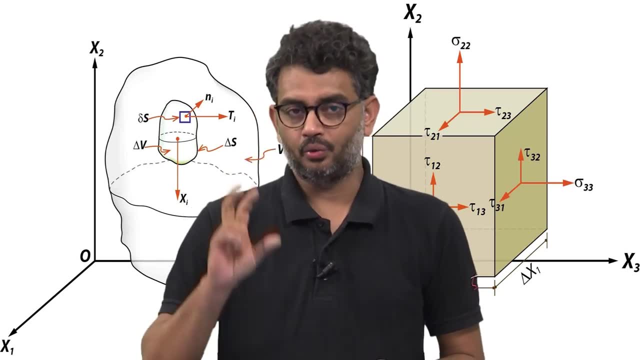 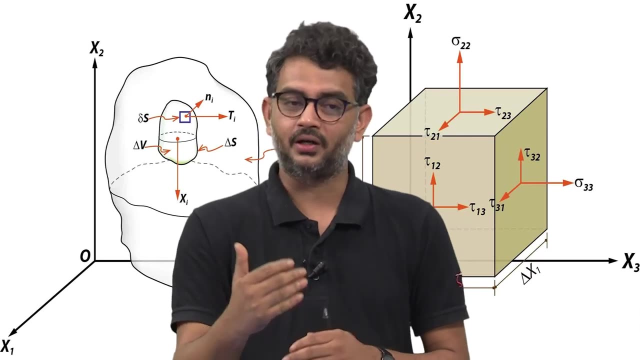 you study the scale of plate tectonics. Now, if you consider the scale of geodynamics, then we consider crust, mantle and core. We hardly consider the fact that crust has different layers, mantle has two different layers, or maybe we consider, but the scale increases. We do not really consider that, whether in 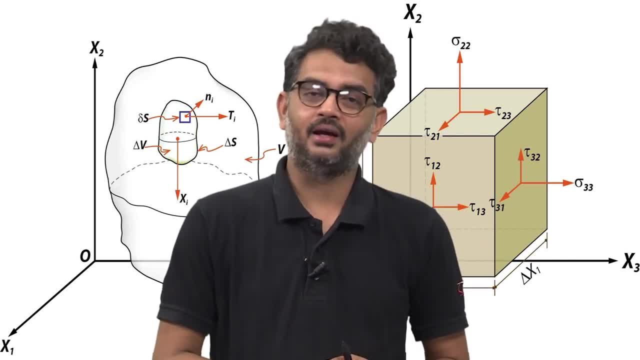 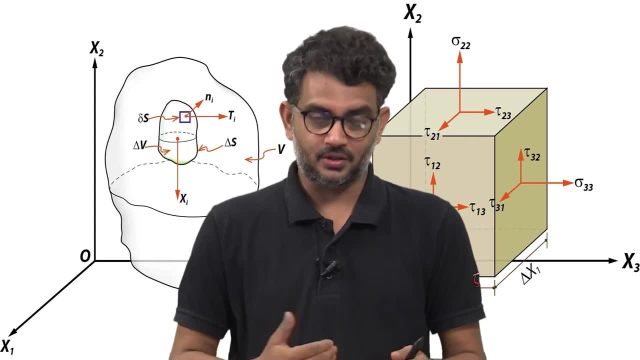 the crust we have carbonates or we have silicates, or whether in silicates we have shell layer somewhere or sandstone layer somewhere. These things do not influence the research of your study. If you would like to study the solar system entirely, then you consider all the planets. 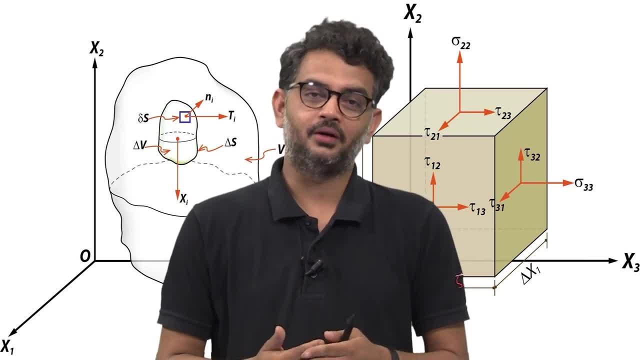 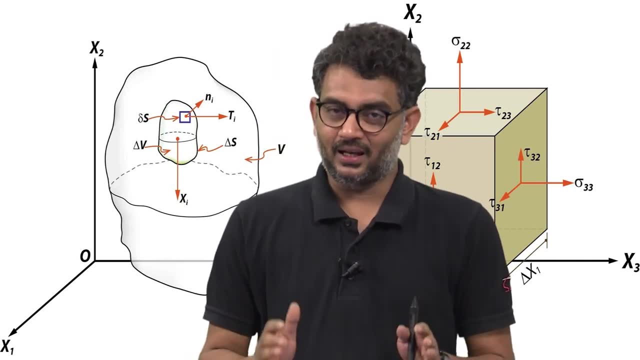 just as a sphere. So there you do not consider what is your core, what is your mantle, what is your crust and so on. So the bottom line is based on the scale you are observing. So scale term is based on the scale of the surface. So scale term is based on the scale of the. 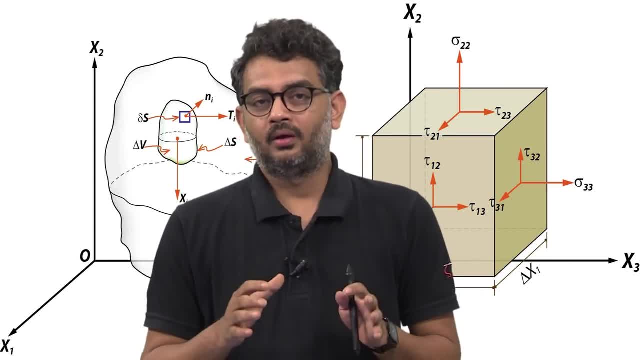 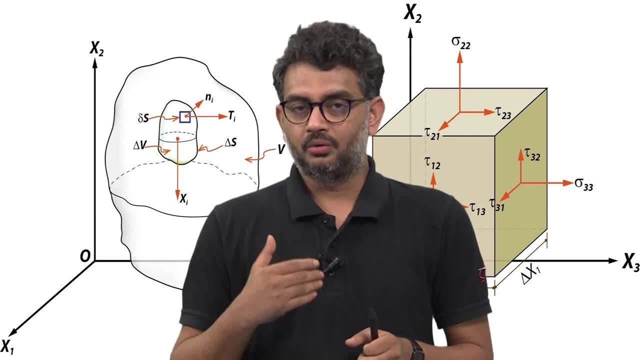 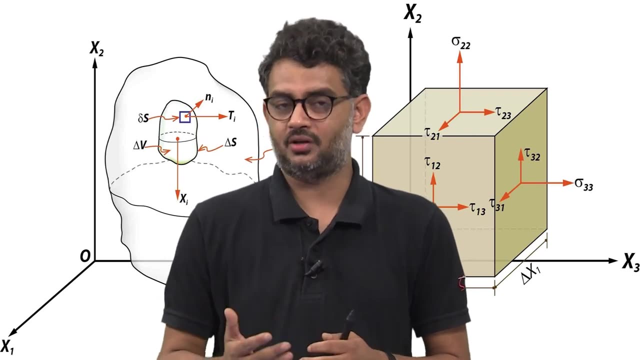 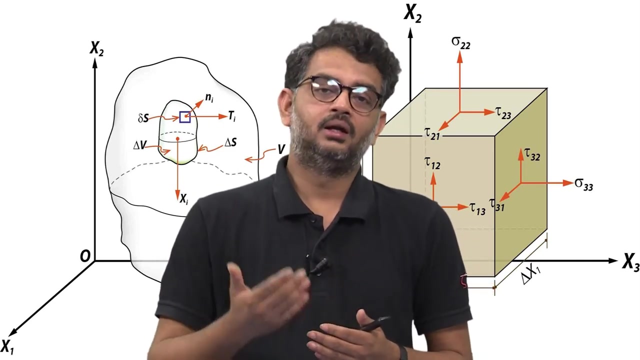 surface. So scale term is very important, as I said in the first lecture. Based on the scale you are observing, or your area or your interest, you somehow approximate some features and you somehow neglect some features. by approximating that, these features, which do not really fit to your scale carrying out or can influence your measurements, or 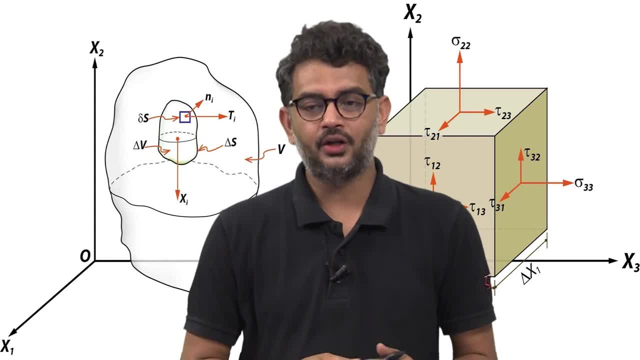 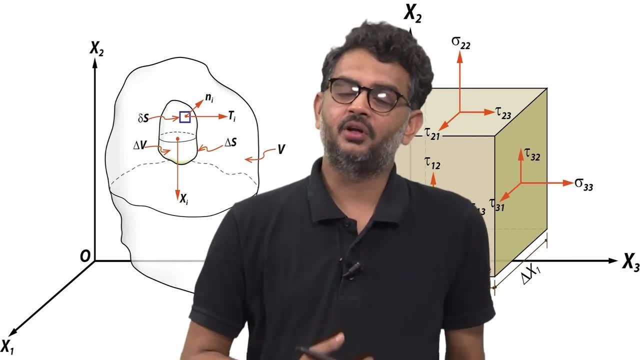 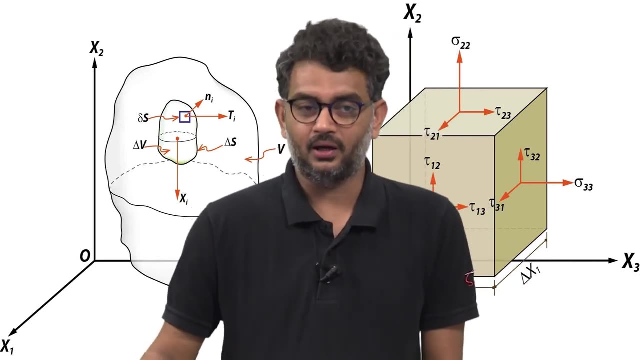 your analysis. So this is the concept of continuum mechanics and we will see that stress and most and strain as well that we have learnt. these are being studied and in the next, after few lectures, we will study rheology. These are subjects which are being studied under the broad umbrella. 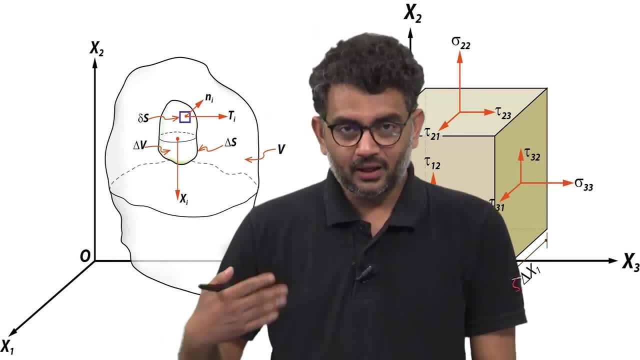 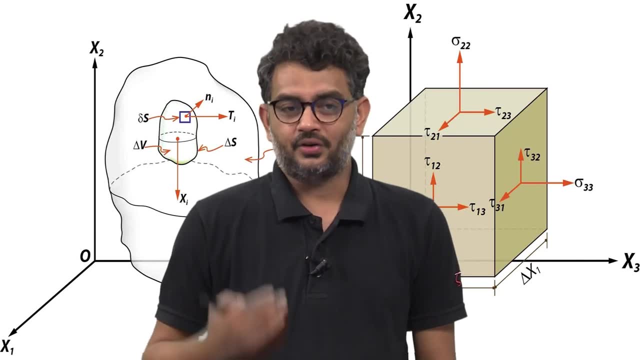 of continuum mechanics. So I hope I can send you the message of why we should. or what is the justification of studying stress, strain and rheology like stress. So I hope I can send you the message of why we should. or what is the justification of studying stress, strain and rheology like 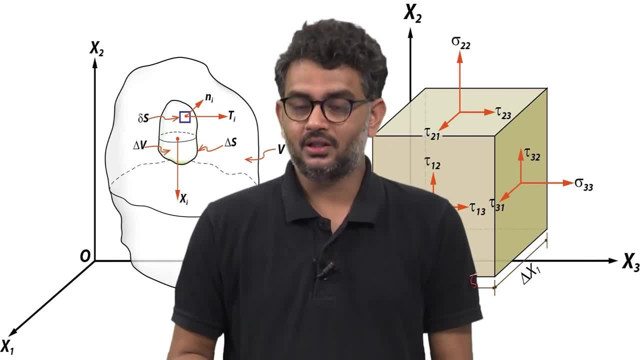 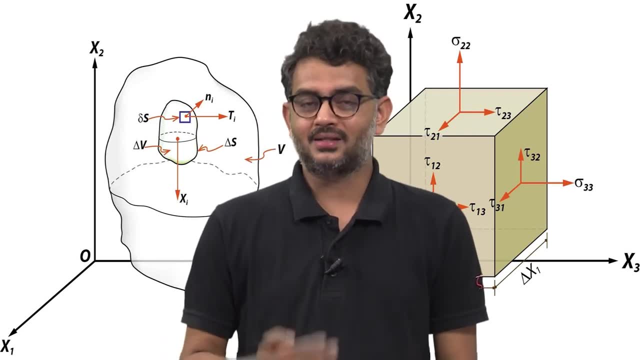 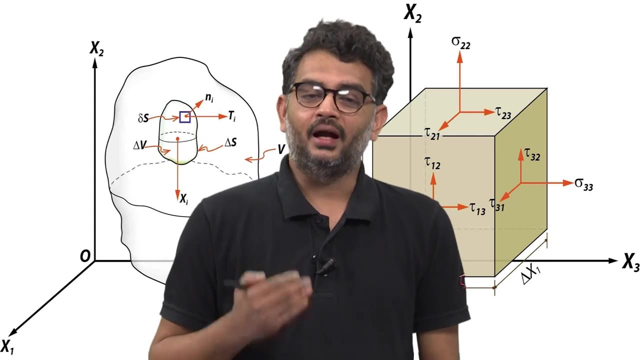 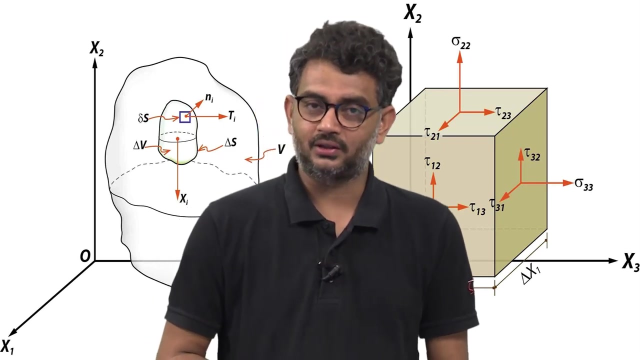 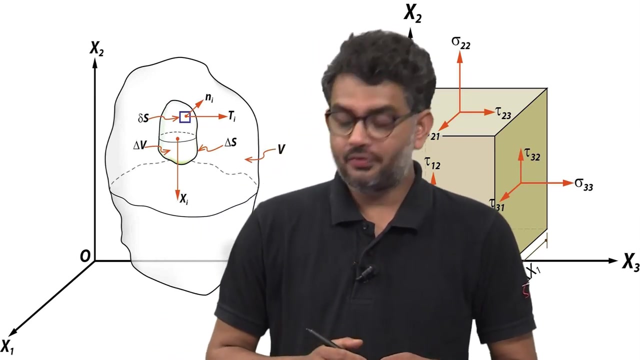 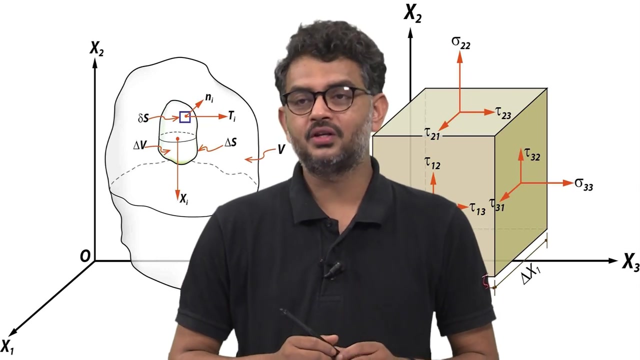 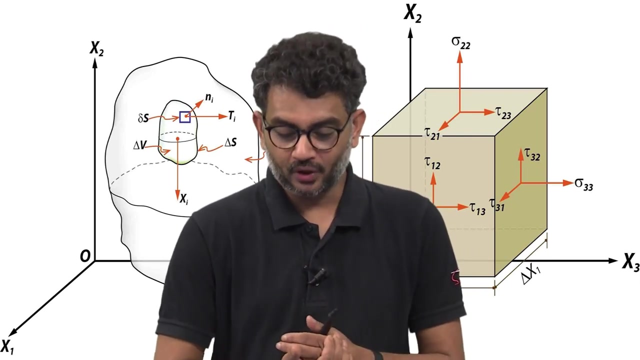 stress And we first get the very basic idea of what is force. Now, if I ask you what is force, then generally the common answer we get that force is a pull or push of a body, or that you apply to a body. So you are pulling a body. that means there is a force, you are 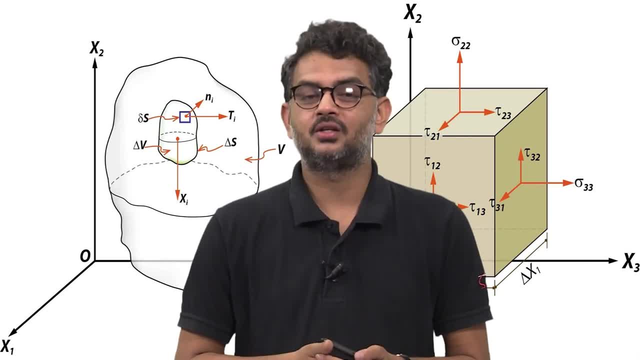 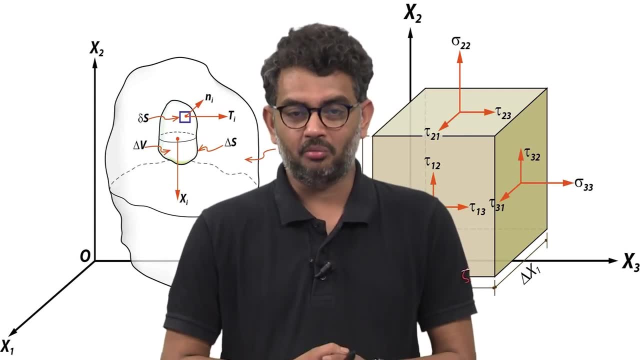 pushing a body, that means there is a force. Now, this is true, but this is not absolutely true in defining the force. For example, I am standing here. apparently no one is pulling me or no one is pushing me, but there are some forces. there is at least one force acting. 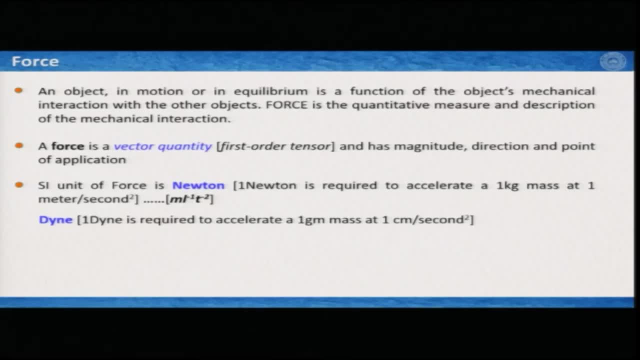 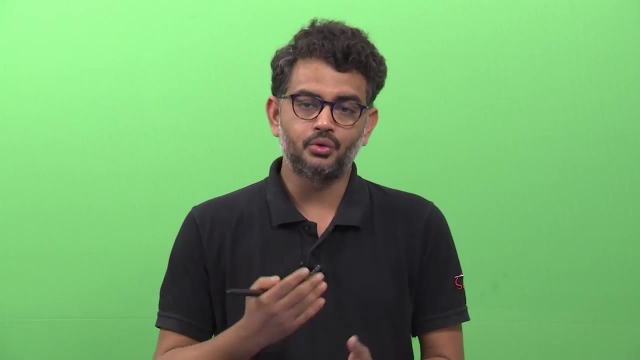 on me. So that is the gravitational force which is going down, and then there is an opposite and equal force which is acting from the ground to me, and that is why I am more or less balanced here. So it is the interaction of the material. 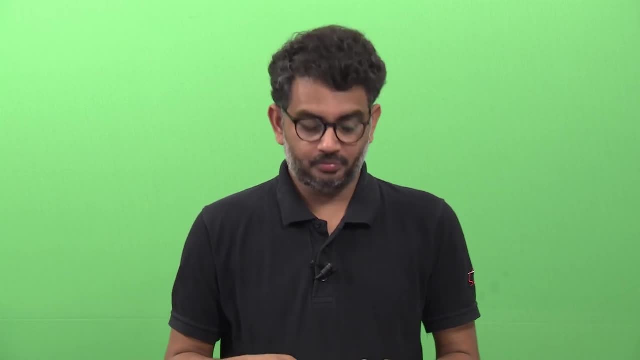 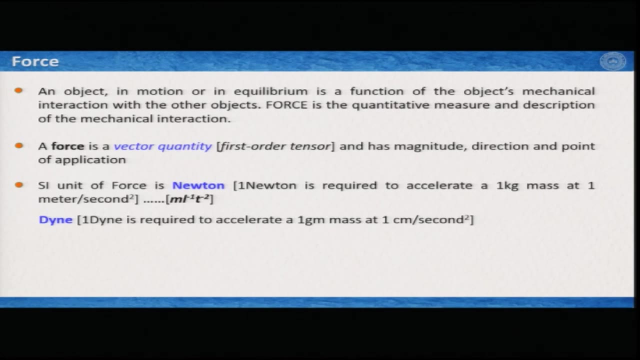 to some object. So we can define that an object in motion or in equilibrium is a function of the objects, mechanical interaction with the other objects. Now force is the quantitative measure and description of this particular mechanical interaction. So that means if you have a 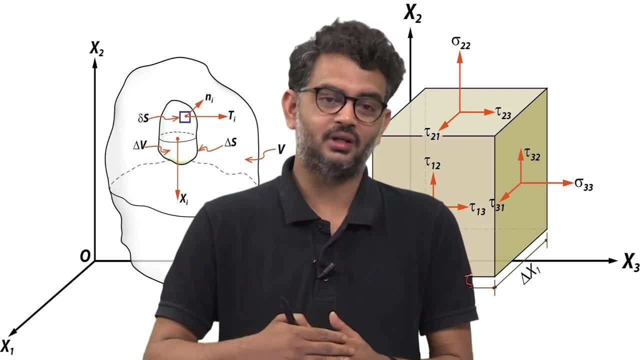 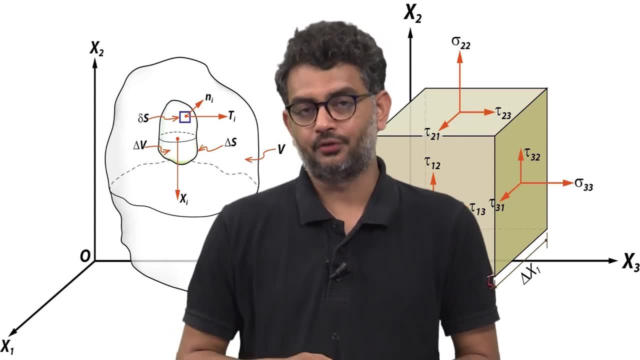 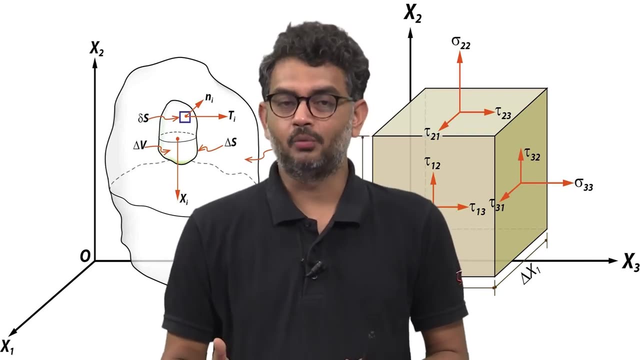 material, then how this material is interacting with its neighbouring or other objects is the study of force, or it is defined as force If you can measure it quantitatively, and that means not necessarily all the bodies have to be in motion to identify or to measure force. Now, force we know from high school. 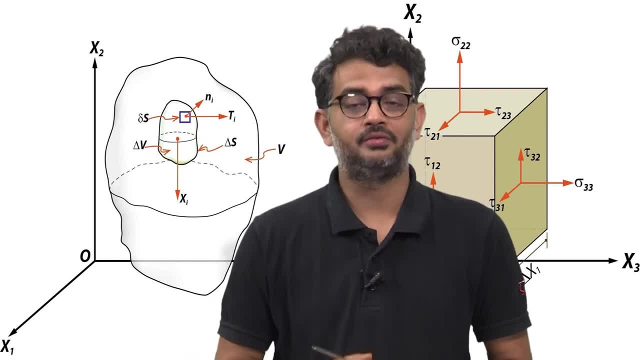 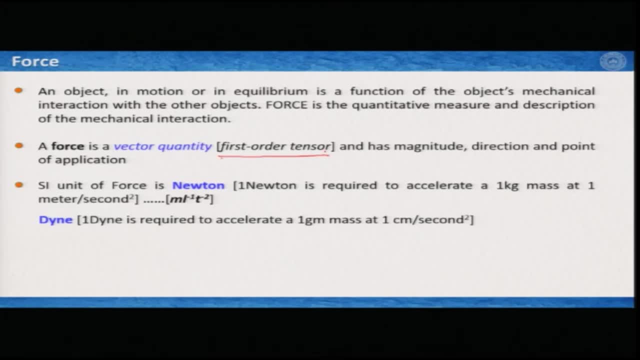 level is a vector quantity. that means it is a first order tensor. Now, this is something a new term may be. you are hearing- we will not go into the very detail of what is tensor, but any scalar quantity. we call it zeroth order tensor. So this is the first order. 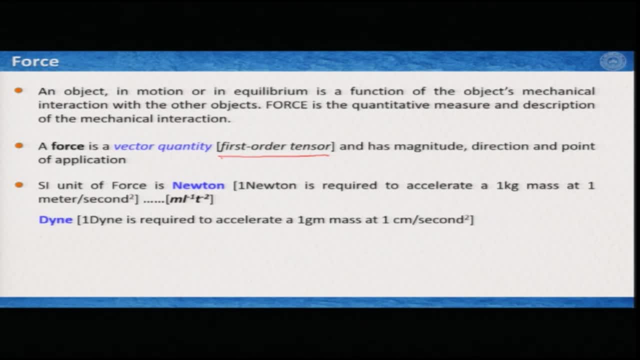 tensor. that means it has zero order, that means it has only magnitude, no directions, nothing. So it is zeroth order tensor vectors. it has magnitude and directions. So therefore it is first order tensor and there are possibilities of some second and third order tensors and 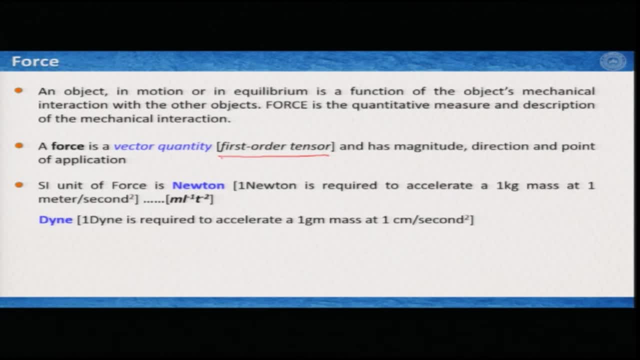 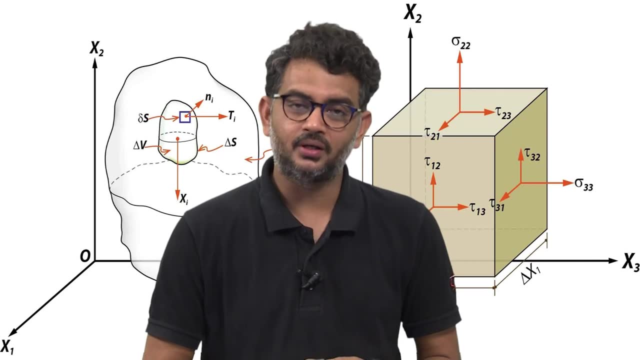 these are not typically vectors or even higher order tensors. We will learn about it soon, but not in detail. but we will just describe what is this. So a vector is generally for first order tensor- let us get into that- only So force, as it is a vector quantity. 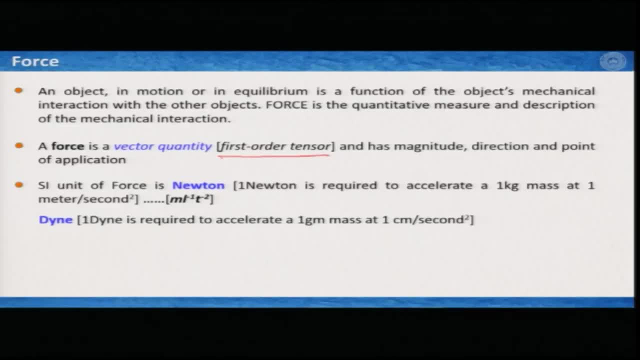 it has a magnitude and direction and point of application. The SI unit of force, you know it is Newton. 1 Newton is required to accelerate 1 kilogram mass at 1 meter per second square And if we see its dimensions then it is M, L prime 1 and T prime 2. that means mass length. 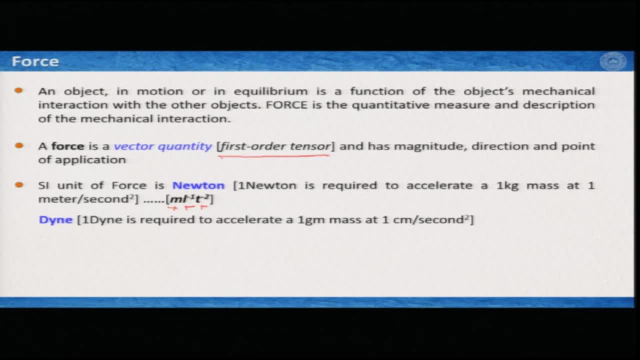 so this is how M L T are considered- would vary when we consider other materials. Then there is also one unit of force that people commonly use is called dine. So 1 dine is required to accelerate 1 gram mass at 1 centimeter per second square. Now to get the concept. 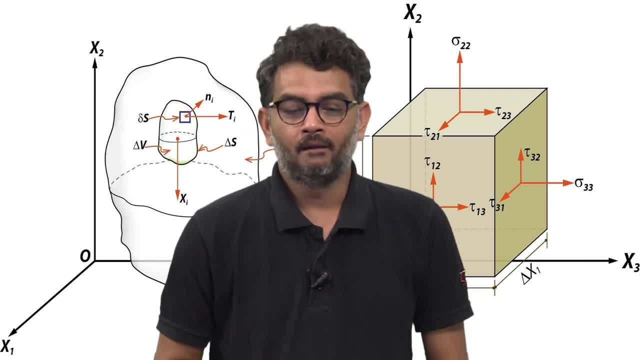 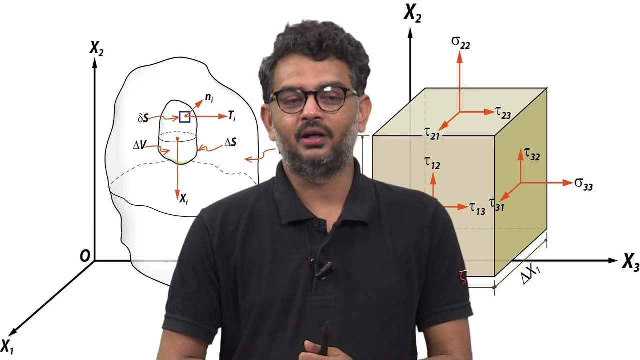 of Newton or just to see that what is 1 Newton? you can actually do it very simply. I just tell you that it is about hundred and Two grams weight. if you keep it and leave it on the earth surface, then you are generating actually 1 Newton force on the earth surface. So you just have acceleration of gravity. 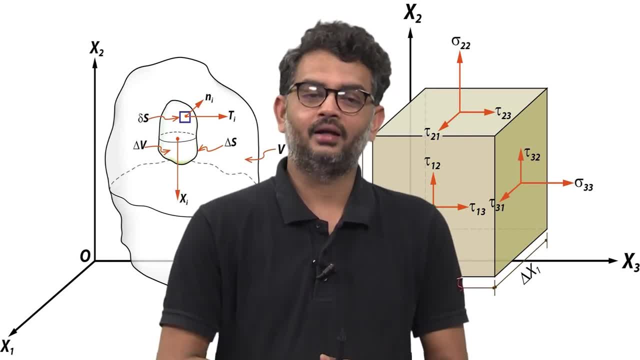 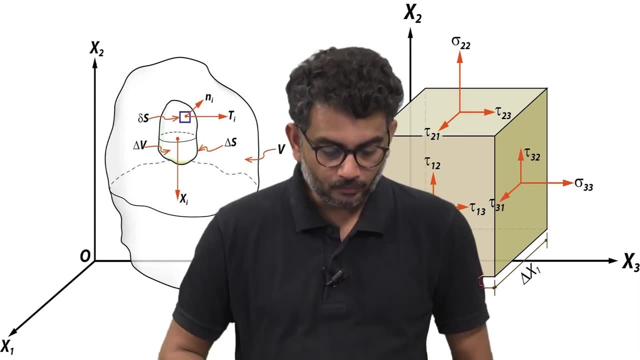 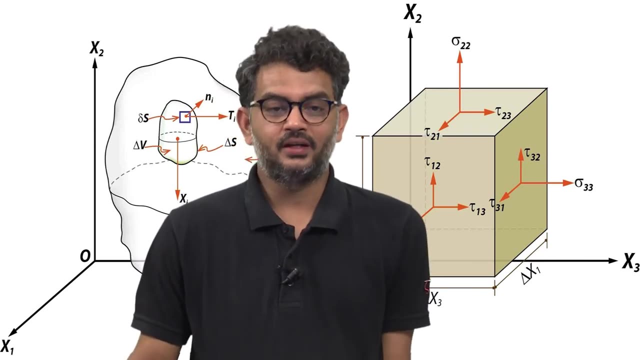 of earth and then you add it to this weight and then you would figure it out that it would. it would come to almost hundred, to grams Now, because force is vector. so you can represent it through a coordinate system in two dimension and 4th dimension and three dimensions. I am. 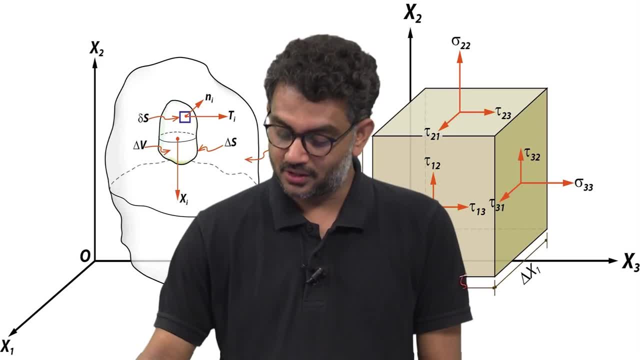 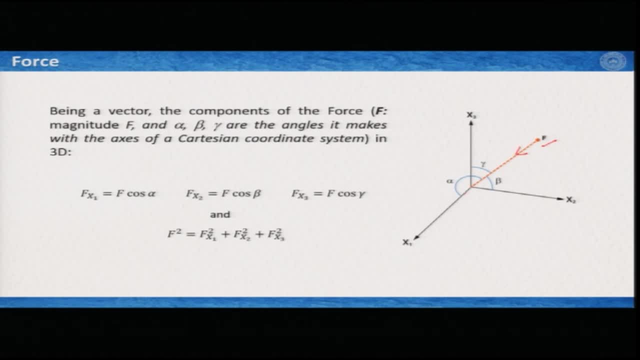 sorry. So what you see here in this illustration. so this is a force, a point which is say, being applied to this direction, to the center of this coordinate system- x1, x2 and x3- and we can resolve this force vector in three different components acting parallel to x1, x2 and x3. 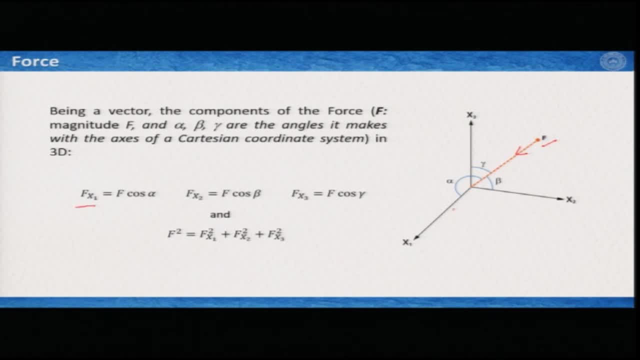 it f x 1 which is acting parallel to x 1 direction, then it is f cos alpha, where alpha is the angle between the force vector and the x 1 axis. And similarly you can have f x 2, where you can represent by f cos beta, where beta is. 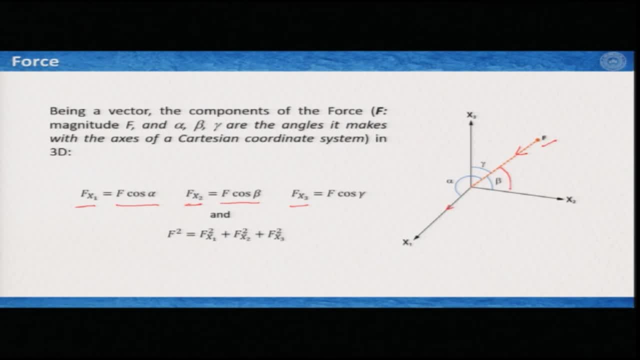 the angle between the force vector and the x 2 axis of this coordinate system and f x 3, where f cos gamma, where gamma is the angle between the vector f and the axis x 3 of this Cartesian coordinate system, And because these are related to each other with this equation, 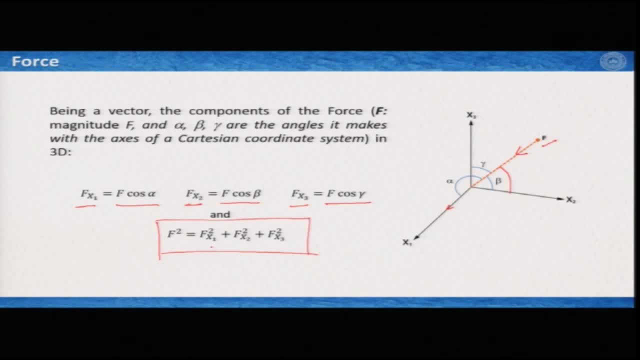 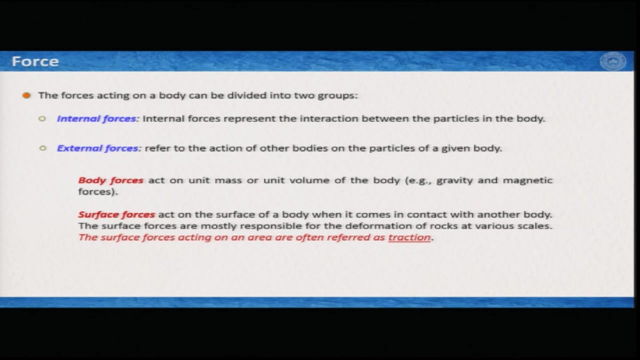 that means a square of this force vector would be sum of the squares of x, 2, x, 3.. Fx1,, Fx2, and Fx3. This relationship holds good. You know it from your high school level. Now there are classifications of forces. There are different classifications, but in 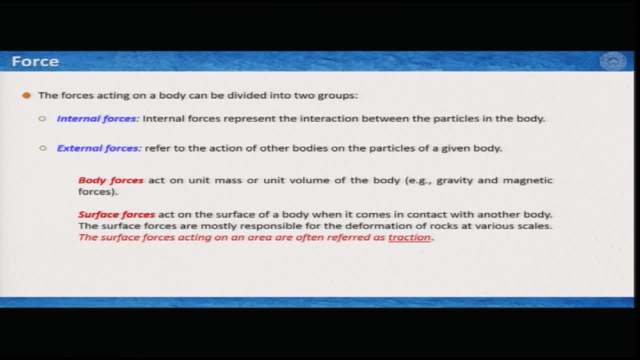 general forces when it acts on a body. we can basically divide into groups. One group is internal forces and another group is external forces. Now, internal forces is something that you can define it, that it represents the interaction between the particles in the 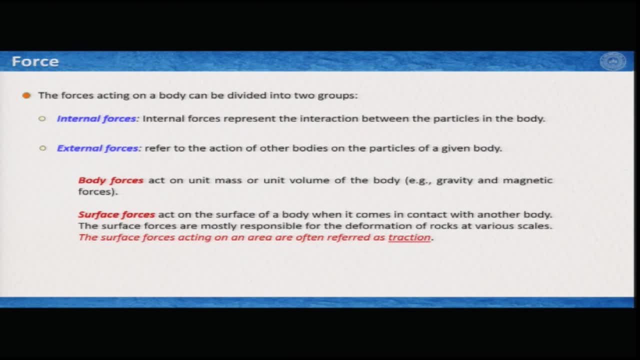 body. So triatomic forces, interatomic forces, inter or intermolecular forces, these are generally considered as internal forces, External forces, on the other hand, that is something when you have interactions of your concerned material on the particle, on the particle. 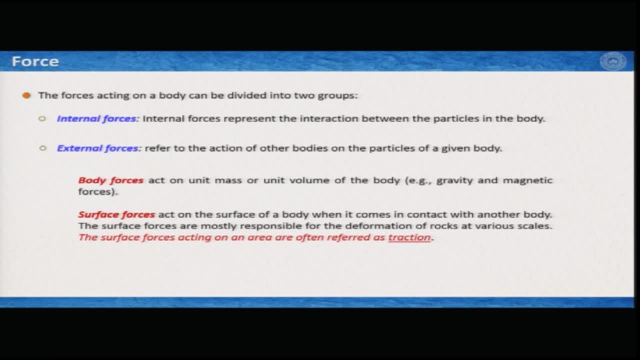 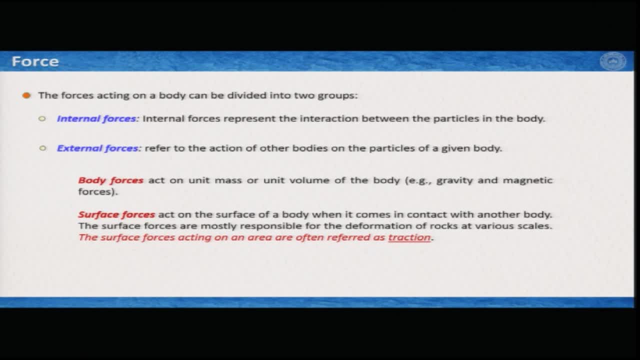 some sort of externally, and this is something we generally consider. And external forces are also classified in two different ways or in two different subsets. One set is body force and another set is surface force. Now, body force is when it 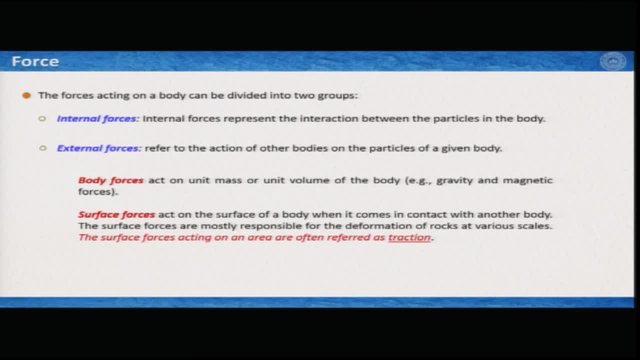 acts on unit mass or unit volume of the body And in the context of geology or structural geology in particular, gravity or gravitational force is the force that you can consider as body forces. Then there could be the magnetic forces that also are a type of body force. 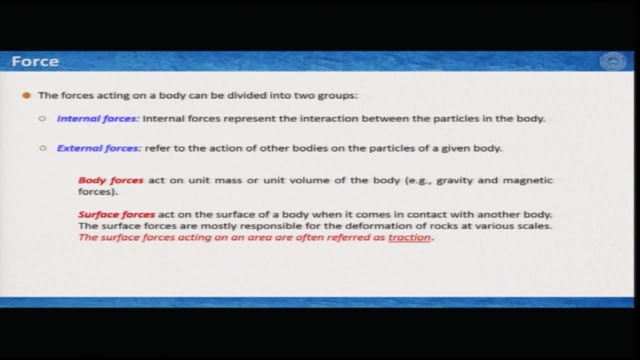 Now, surface force- that is something very important to us- is defined as the surface forces do act on the surface, The surface of a body when it comes in contact with another body. the surface forces are mostly responsible for the deformation of rocks at various scales. So you need a contact. 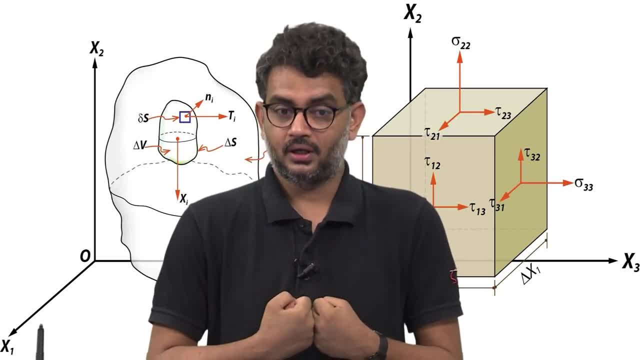 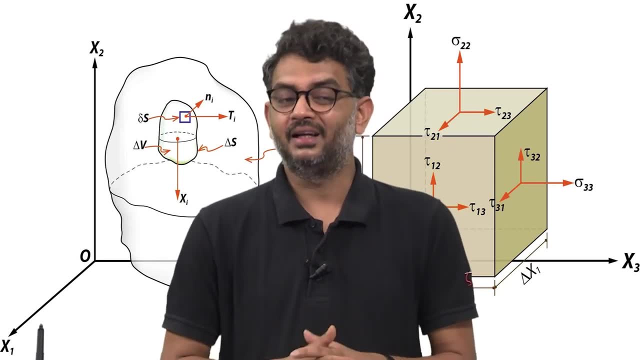 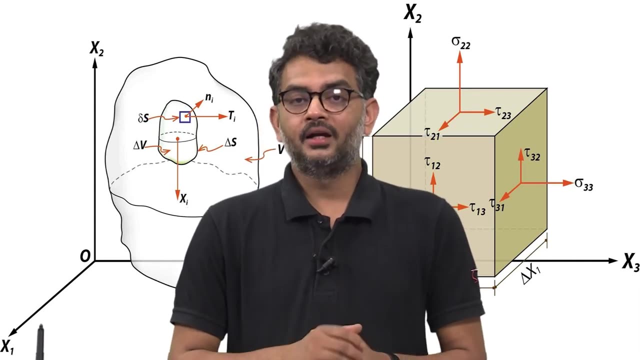 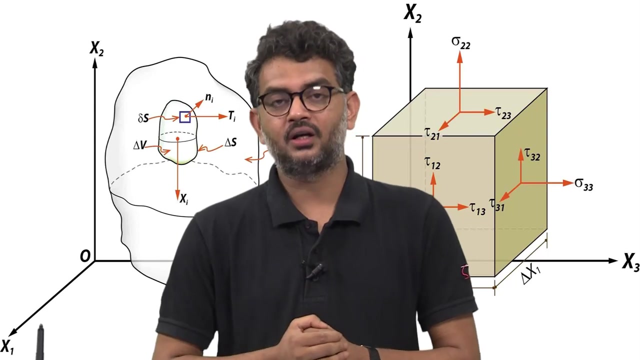 to have some sort of surface forces, Otherwise your body will not deform. and if there is no distortion, no deformation, then you are not dealing with surface forces. You probably are dealing with body forces or some other forces. Now, surface forces, because it has to act on an area of the object you are considering. 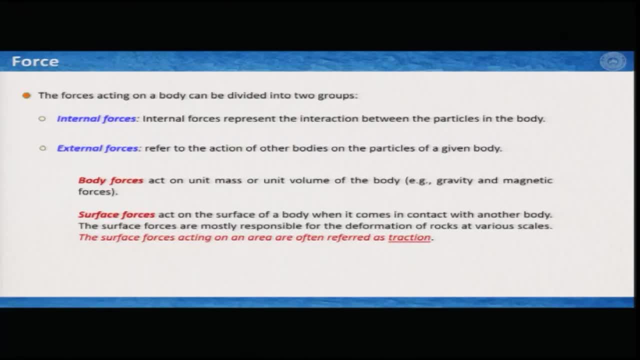 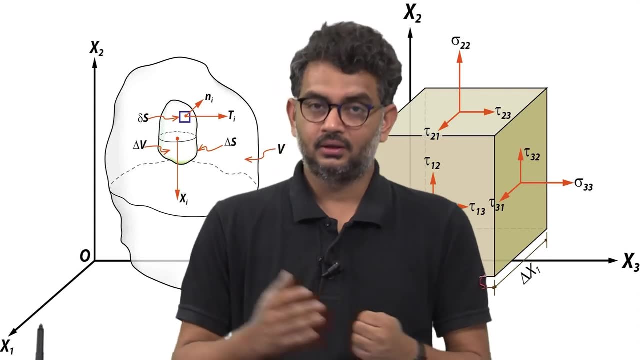 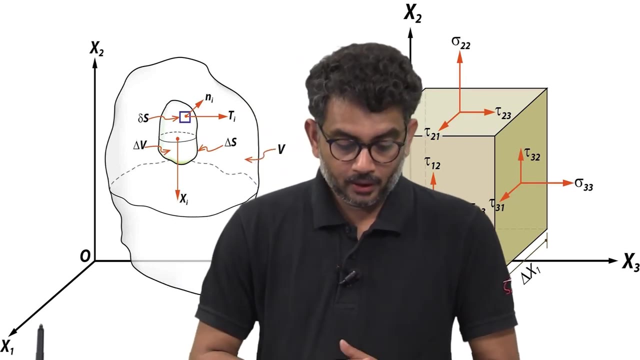 with. so this is often referred as traction. So we will see what traction is, that when a force acting on an area. sometimes we call it traction. You remember this term? we will use it soon, So let us have a look first. 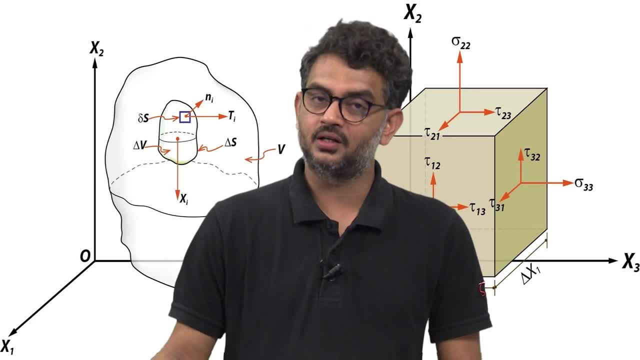 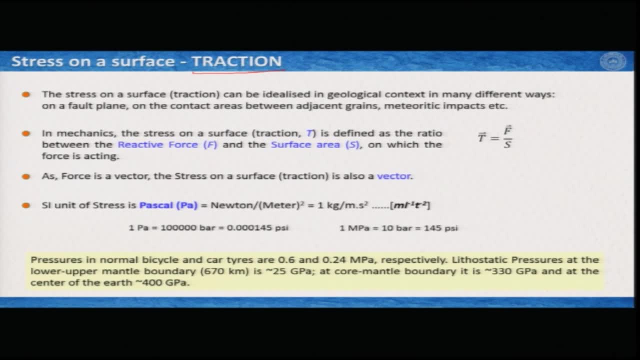 So on the stress term, when it is acting on a surface or we define it as traction, The stress on a surface can be idealized in geological context in many different ways. For example, when you have a fault plane, then two planes are moving past each other. 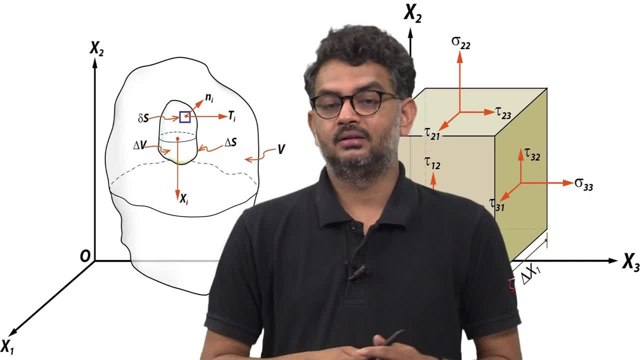 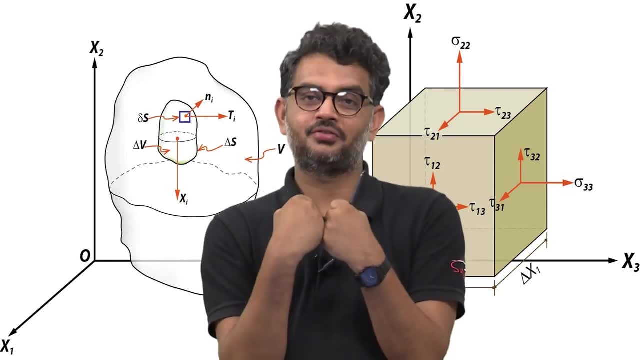 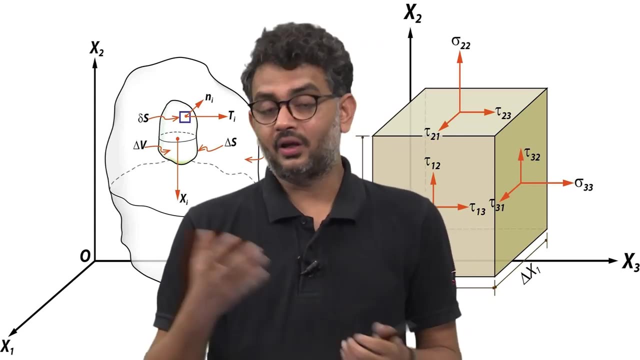 keeping a contact. or you can imagine that two grains are in contact in a very micro-scale and one grain is transferring its stress to the neighboring grain. That means it is generating a traction at the grain boundary. You can consider of meteoritic impacts and 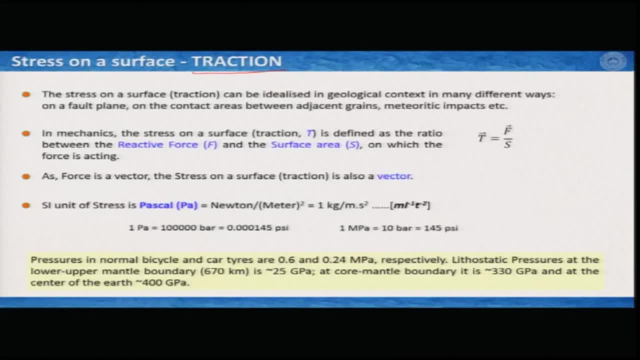 so on. These are some very visual examples, but wherever there is a deformation, there is a traction. You can think this way. So the definition of stress generally, we say, or we commonly say, that what is stress? Force per unit area. You are right. 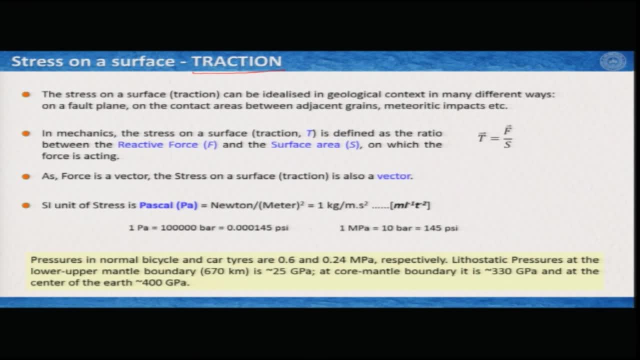 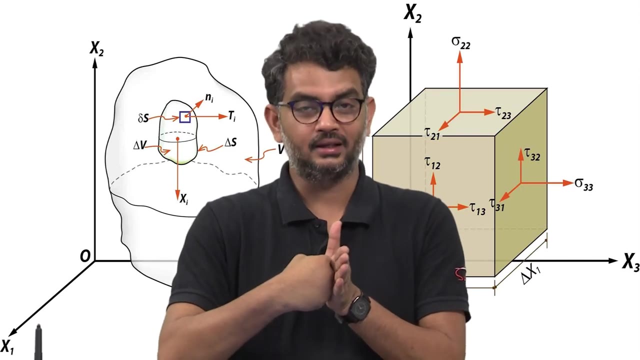 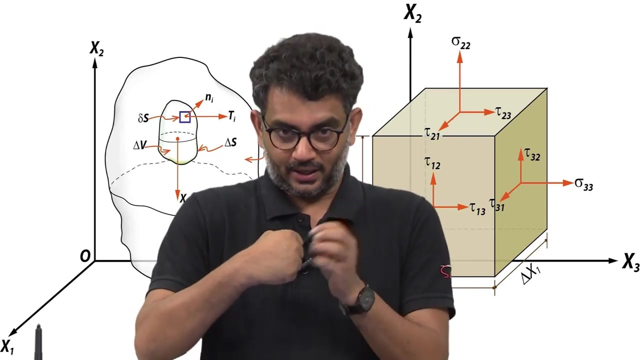 But that is not absolutely true. It is actually the reactive force per unit area. That means if I apply a force here and if I calculate, if I know the magnitude of this force, that I am pushing my left palm with this right hand punch, then if I apply, take this force. 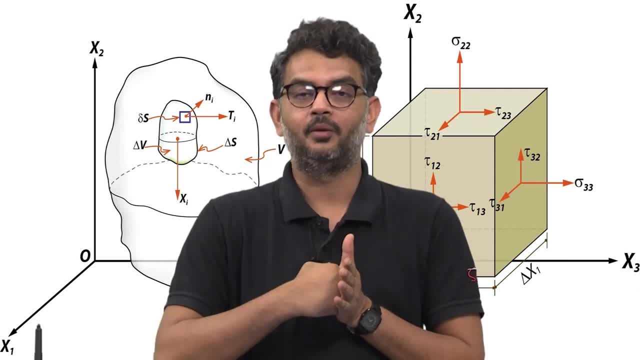 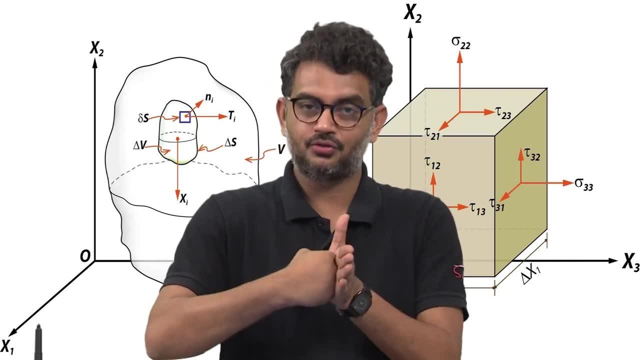 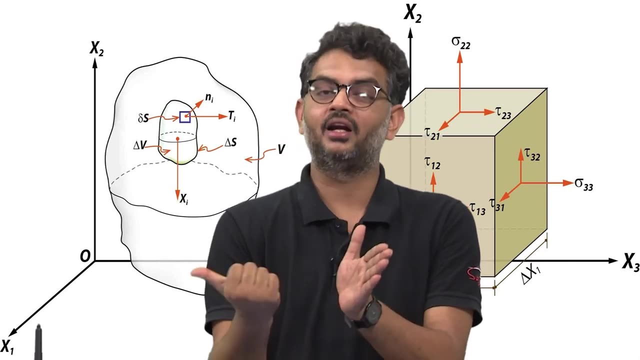 and divide it by the area of my left palm, I certainly get a value. but that is not stress. Stress is I am applying this force and my left palm is working or pushing with an opposite and negative force To the force. 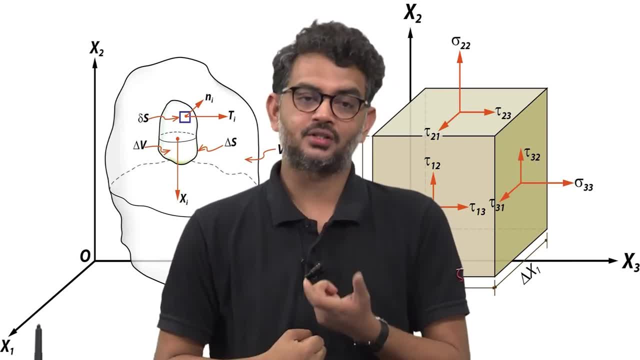 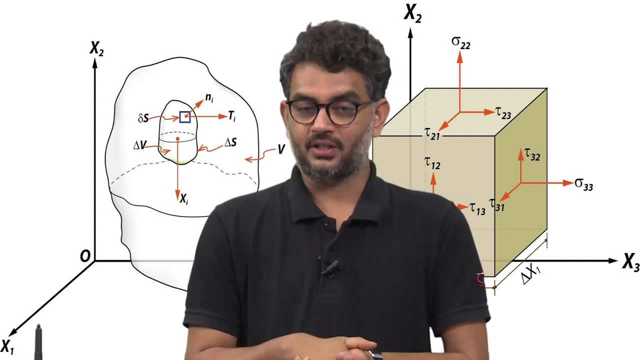 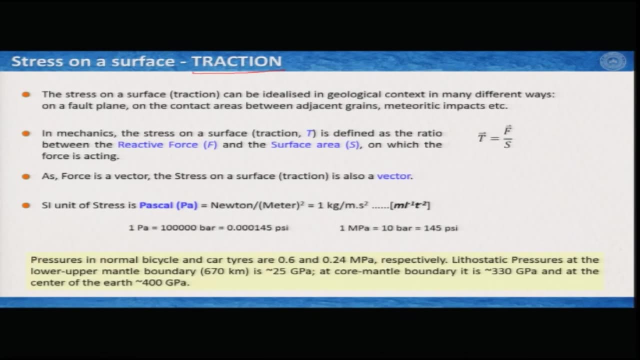 is being applied by my right hand. And this force is reactive force, It acts following the Newton's third law And this force, divided by the surface area, is the stress. So this is the stress generally defined. So the stress on a surface, or you can say traction, 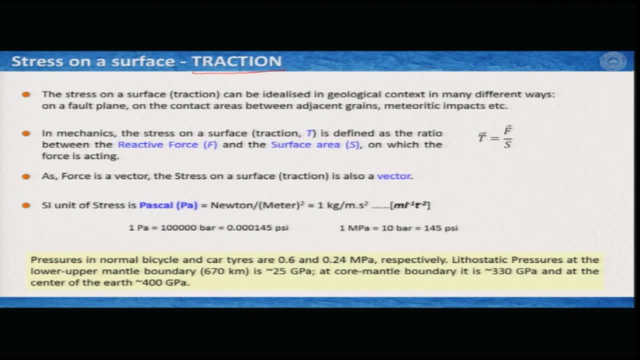 will define it as t, as defined as the ratio between the reactive force f and the surface area s on which the force is acting. So, therefore, we define that. this is what is your reactive force. It is a vector force, Then this is the area you, you would like to work with. 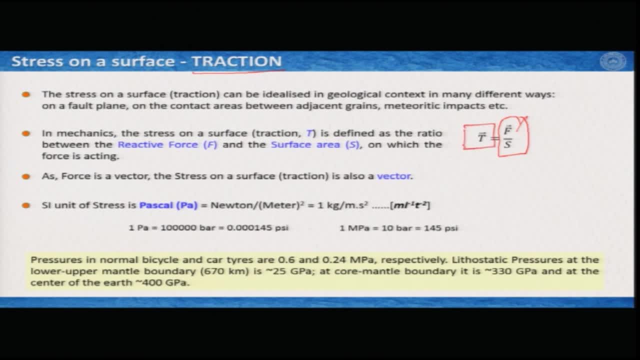 So this T is a stress or the traction Now, because force is a vector, so the stress on a surface or traction must be a vector as well. Now, because we are adding some area or dividing the Newton by area, then unit of stress should be Newton per meter square. 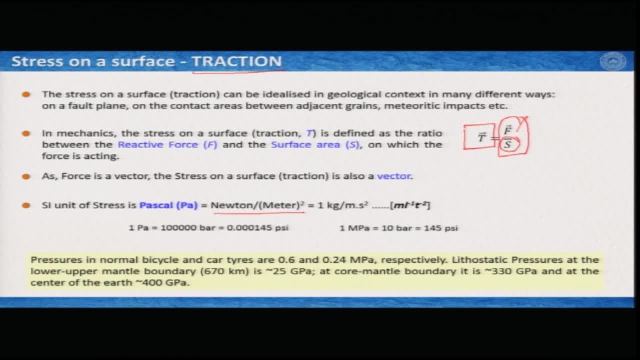 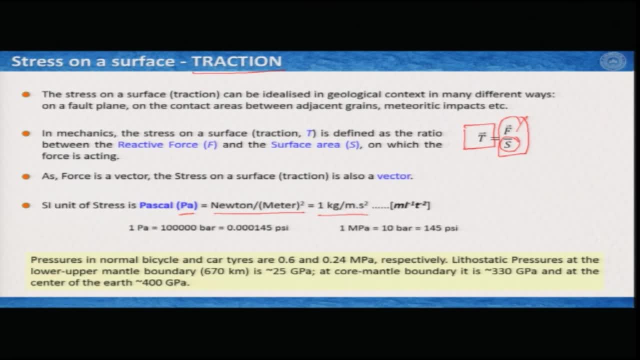 you can, you can expand it. So it is one kilogram per meter per square and the dimension here changes to m, l power minus 1,, T power minus 2.. Now there are many other units of stress. sometimes we also call it pressure in in the context. So one P Pascal is equivalent. 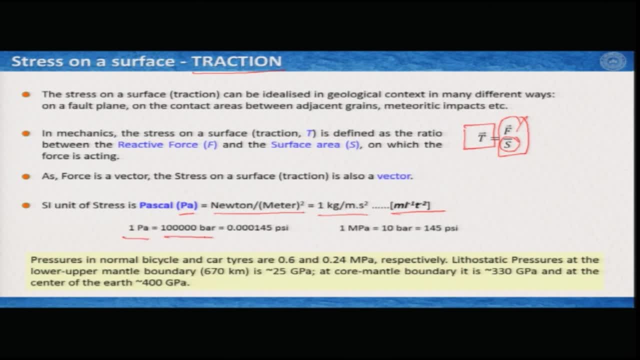 to 10 to the power 5 bars. Now this 10 to the power, 5 bars, that means 5 zeros after 1, and this is about 0.000145 psi pound per square inch And 1 megapascal, therefore 1. 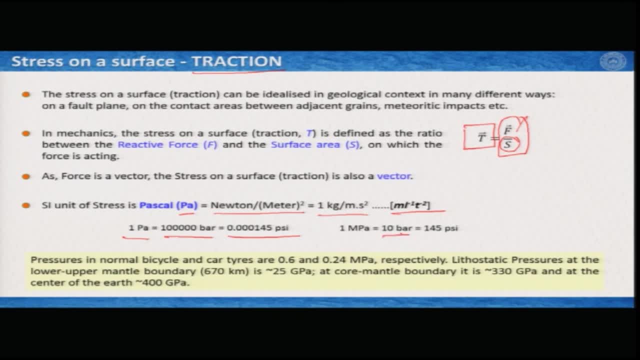 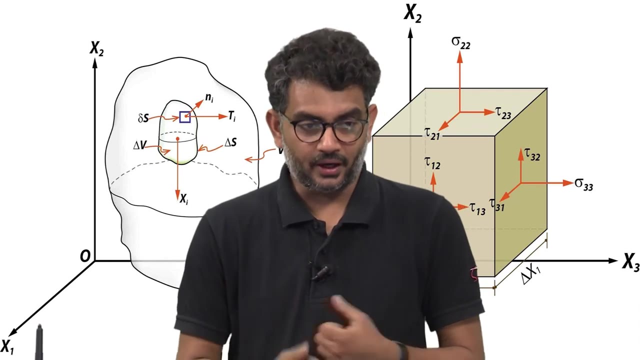 into 10 to the power. 6 pascal is equivalent to 10 bars and 145 psi. Now, what is 1 pascal? or what is 1 megapascal? How much it is? I give you an idea, or it is written here you. can read The normal bicycle that we ride every day. the tyre of these bicycles have a pressure So you have to pump it. So the general range is mostly 0.5 to 0.7 MPa in a normal bicycle tyre. In a car tyre it goes to 0.24 megapascal or 0.3 megapascal maximum. 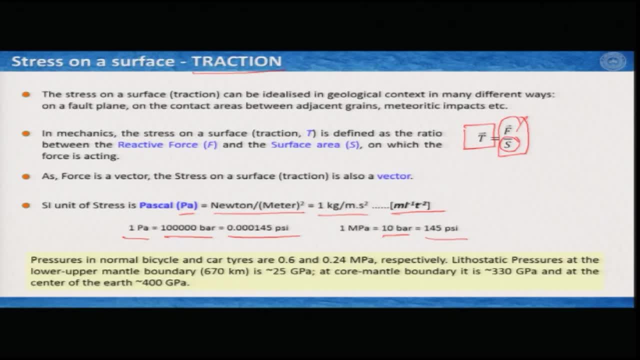 but that is in a very rare case. So the pressure on the bicycle tyre is 0.68 megapascal and the lithostatic pressure at the lower upper mantle boundary, which is around 670 kilometres down from the surface, is about 25 gigapascal. That means 1 MPa. 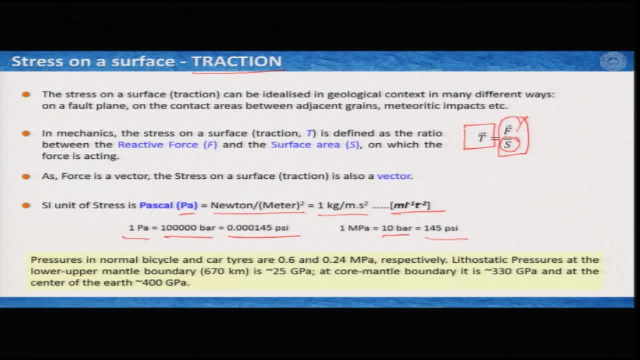 multiplied by 10 to the power 6 multiplied by 25 gives you the gigapascal At core mantle boundary it is about 330 gigapascal, and the centre of the earth it goes close to 400 Pascal, where the temperature is close to 6000 or 7000 degree centigrade. So this is. 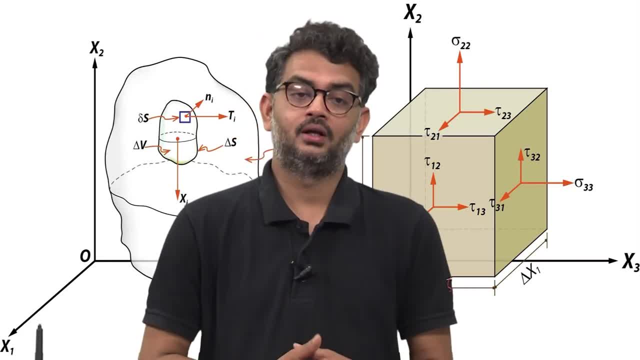 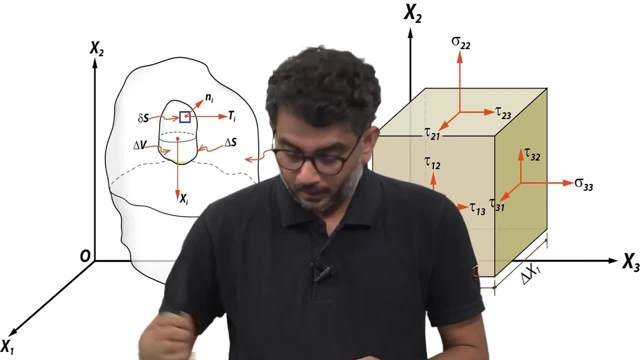 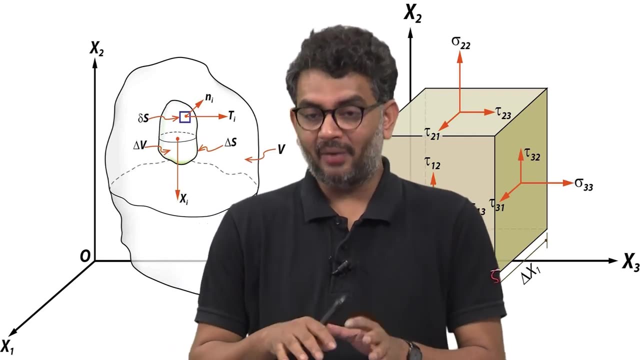 the range of pressure, or this is the magnitude of the pressures that structural geology, tectonics or geodynamic people think and work with. So we will look at now that how to mathematically describe the stress on the surface element. but before that we will take a break. We will 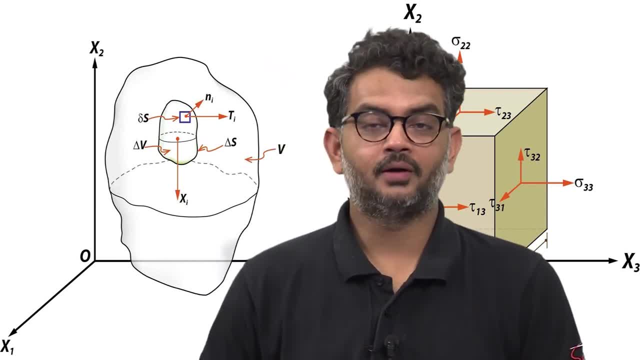 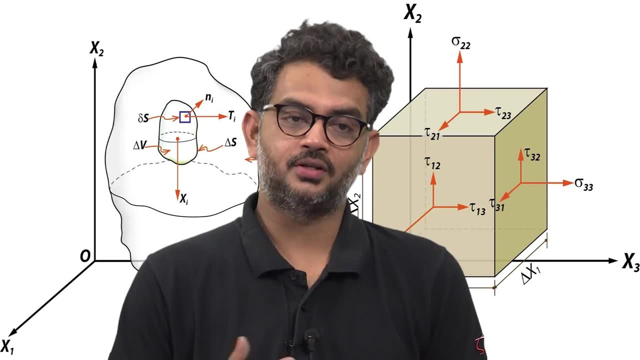 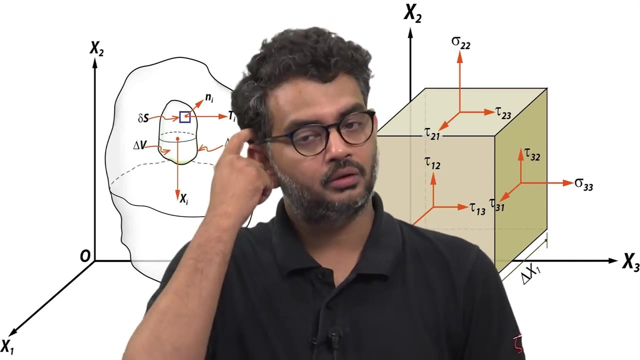 continue this lecture. in the next segment We will come back. So in the previous segment what we learnt that what is stress on a surface, what is its dimension, what are the units and more or less we have an idea that what is mean by stress on a surface. Now, in this segment, we will learn mathematically. 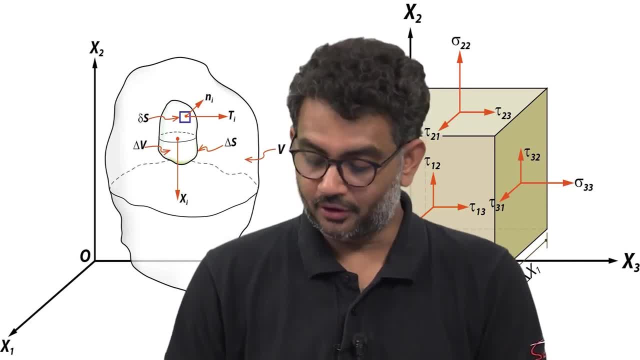 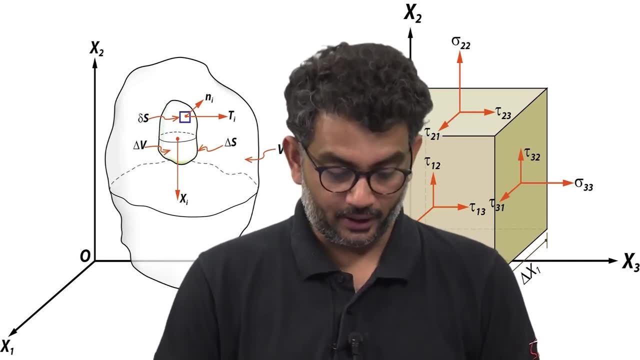 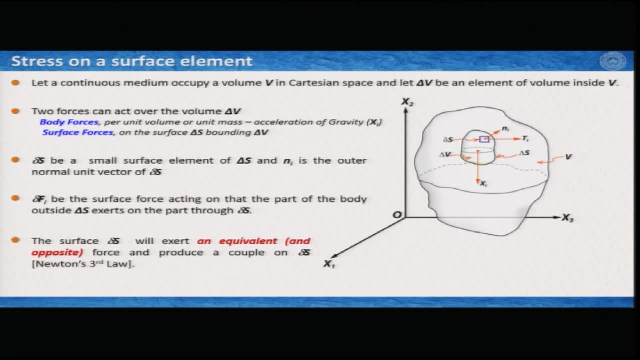 how to express what is stress on a surface, and for that we will consider some sort of approximations under the broader umbrella of continuum mechanics. So, stress on a surface element, to consider that, let us consider a continuous medium which is occupying a volume V, which is this larger area that you see, this one. So this, 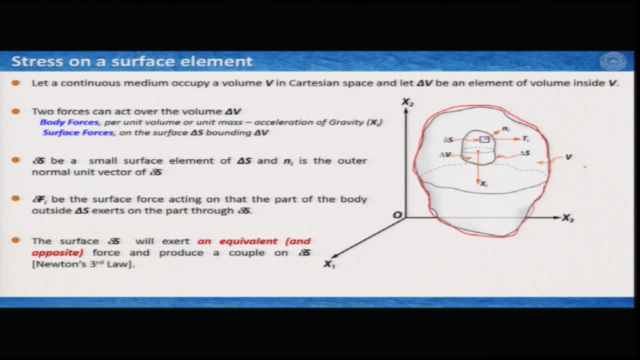 is volume V In Cartesian space and within this you have a very little element, volume element, which is delta V, inscribed in the volume V. Now, if we consider this volume V- now why I am considering this, I am considering this entire. V is a very large body and it is a continua. 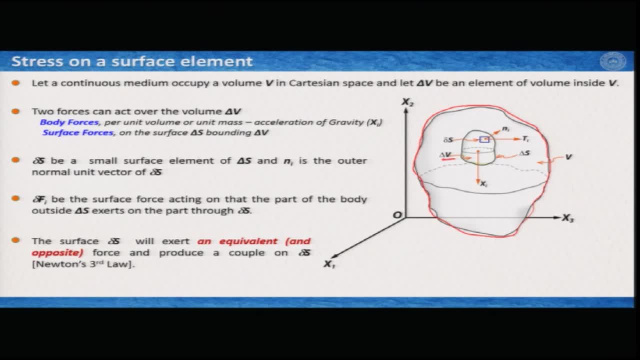 and within this continua, I am considering a very small volume. Now, if I consider this very small volume del V, then, as we have learnt, the two different forces would apply on this. One is body force, which is acceleration of gravity, which is x, i, and then surface forces that must act on a very small surface. So let us consider 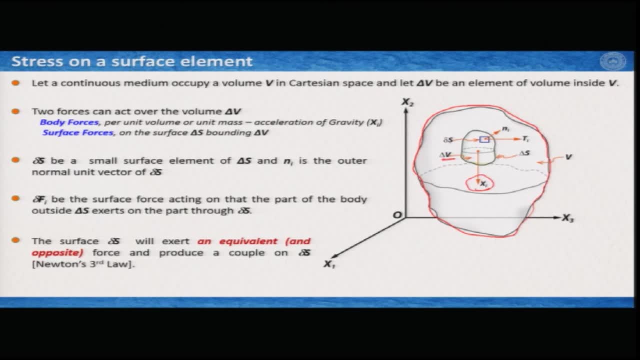 that this is del s? el f seems to be the being that When you consider this total volume del V, you see that this very small surface, which is a very small volume, It is about this volume which is acting, which is acting for我是 acting of this. So now you can engineer this, now how you sort what. 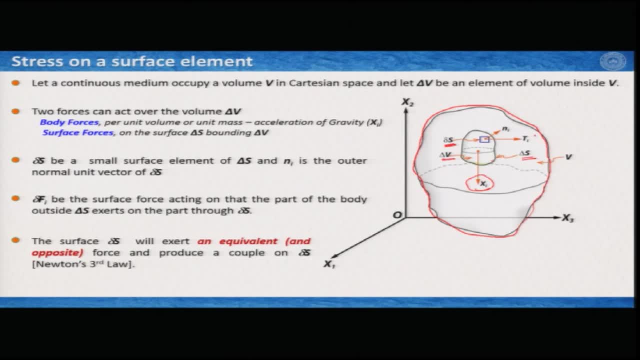 is acting for this volume del V? n In the zones they happen to be not between the zone S and also within the zone I change also this volume del V, they of P, s, l, n, f or whatever, or del f i. Now, what is this? i here, Like, as we said, this n? i n, i is the 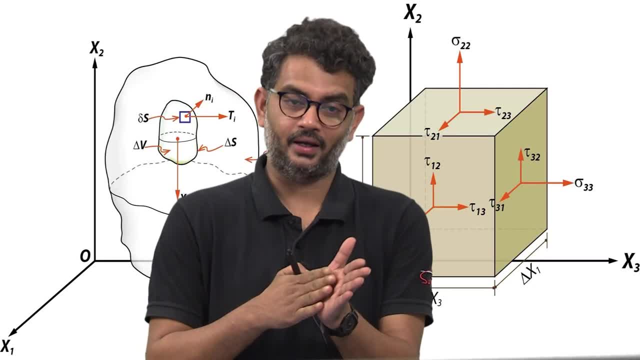 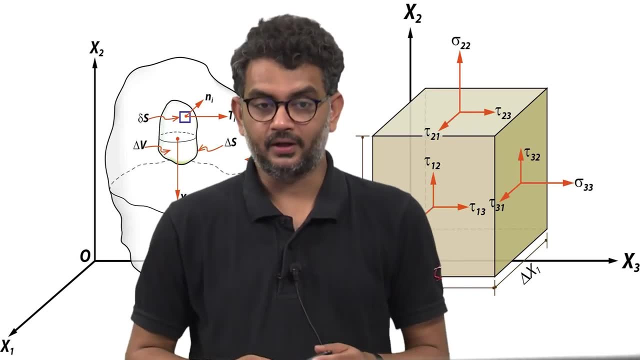 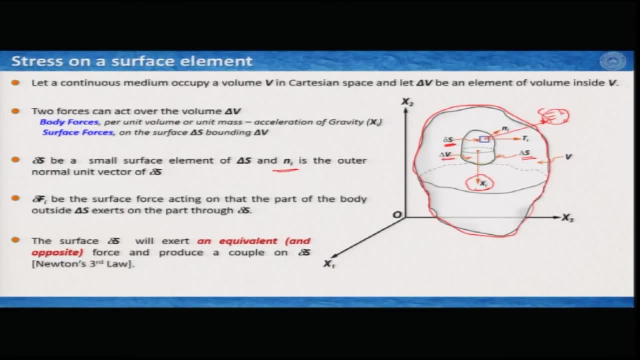 unit normal vectors. So if I consider any surface or any plane then it must have three unit normal vectors parallel to the coordinate axis right. So if I have this very small area and then this del f, i is the surface force acting on that very small area del s. 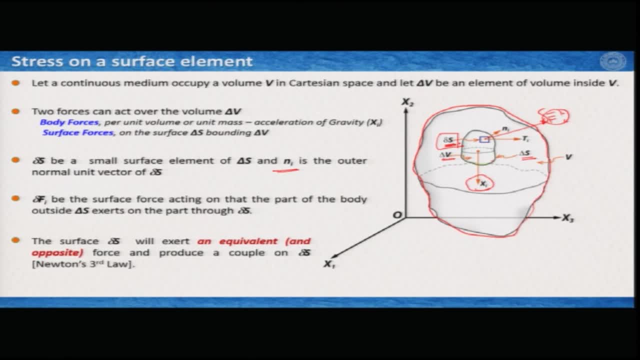 of this body, then this little blue surface area would react to this force del f i, So it would exert an equivalent and opposite force and it would produce a couple. Now I repeat that I have a large volume, v. within this large volume, I have a small volume, which 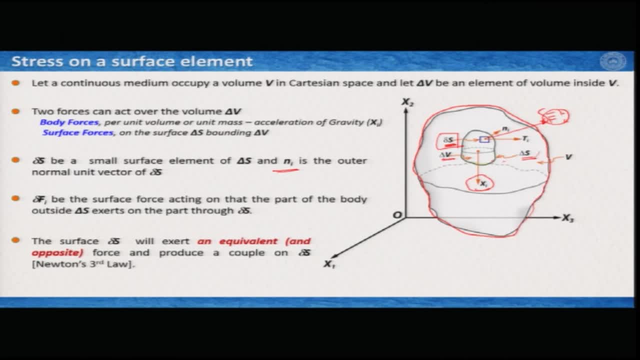 is delta v, which has a surface area delta s, and within this small area delta s we have a very small area del s. So the force is acting and because the force is acting on that little surface, it would exert an equivalent and opposite force and produce a couple on the surface del s from. 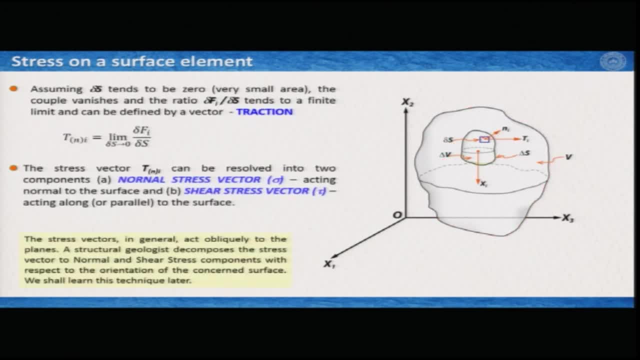 inside. So now, if we considered del, s tends to be zero, that means it is a very, very small area, and then the couple vanishes and the ratio del Fi and del S tends to be a finite limit and can be defined by a vector which is traction. 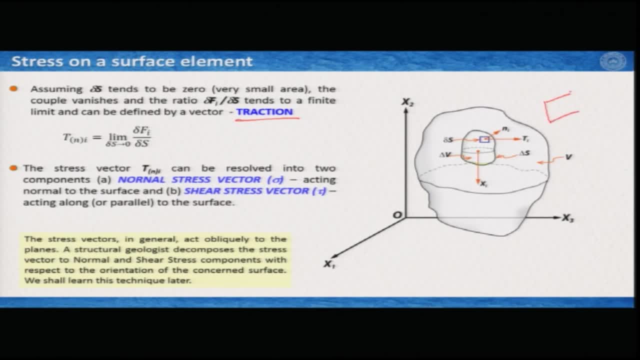 Now, by doing this, that means I have a very small area. I am applying a force, So we are getting an opposite force on this same point from the other side, and this is del S, this is del Fi, So if this area goes very small. so, therefore, I have an area which is 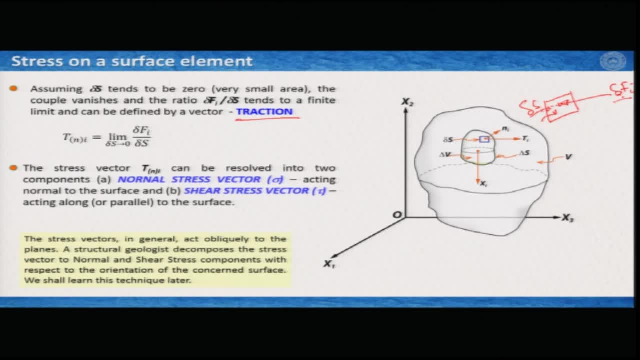 del S and I have a force acting on this, del Fi, and if I reduce this area, that means the area tends to 0, then I get some sort of a very in a very small area, the stress or the traction. So mathematically we can define it this way, even if you not consider this strange mathematical. 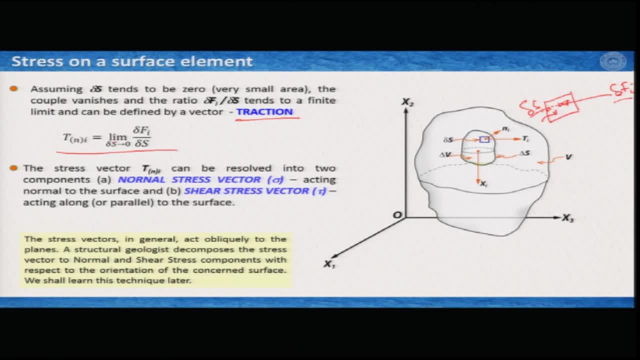 notations n and i. So traction is equal to the limit. where del S tends to 0 is del Fi divided by del S. So this is the mathematical expression of stress on a surface area. Now, this is not really very straight forward expression, as 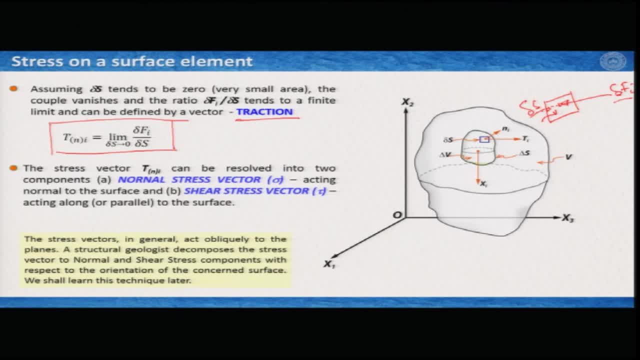 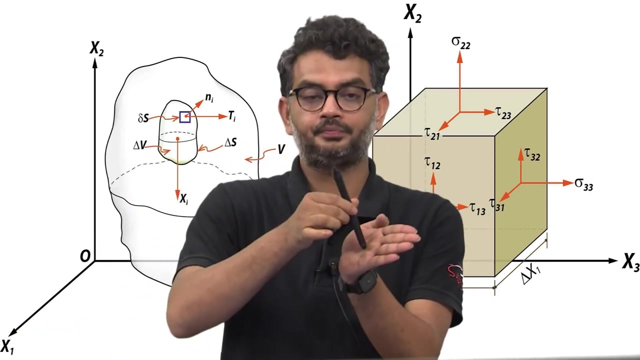 force per unit area or reactive force per unit area. So in stress, in considering stress, this is how we apply the definition of stress on a surface element. Now we clearly see that if we have a surface and I have a force, So we have a force acting on this surface. say, this is how it is working Now, because 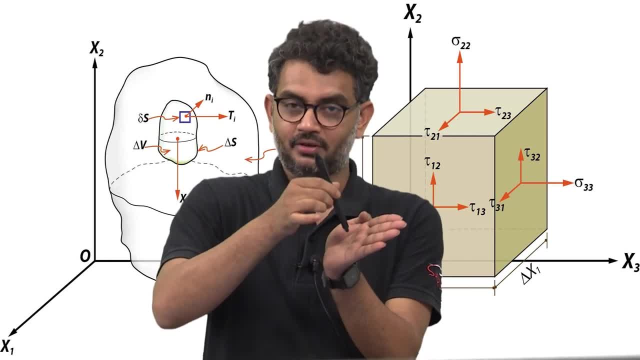 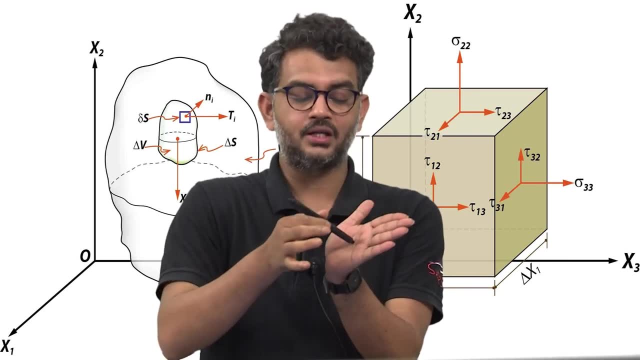 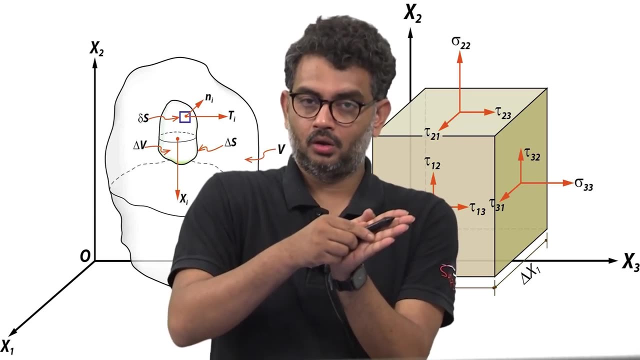 this is a vector. we have understood before that traction is a vector. I can resolve this vector one way that is perpendicular to this plane and another way parallel to the plane. The force vector, or the component of this force which is perpendicular to this plane. 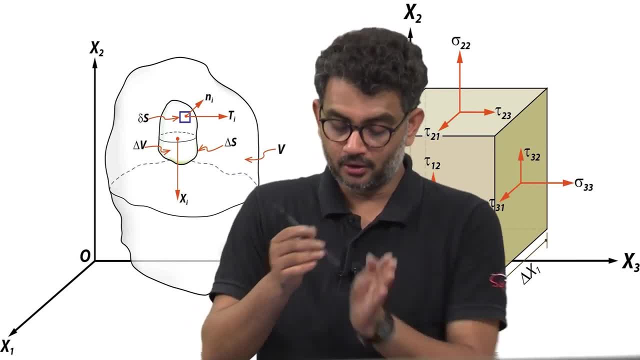 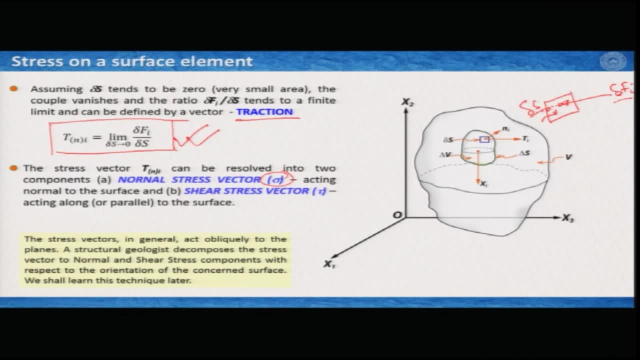 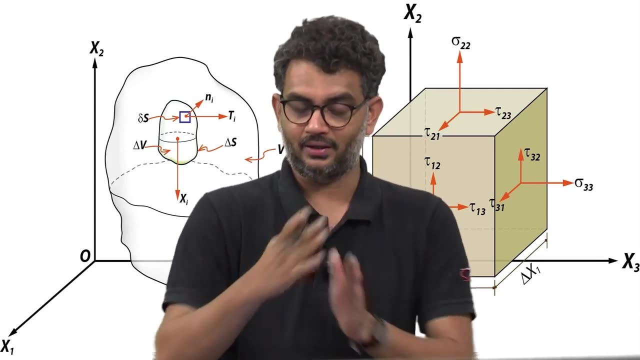 is known as normal stress vector, or we define it or mathematically write as sigma: that acts normal to the surface and there is a force that acts parallel to force component. we can resolve that acts parallel to the surface and this is known as shear stress vector, or 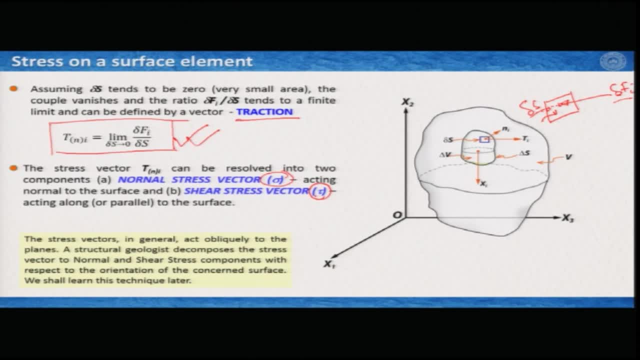 mathematically, generally written as tau, which acts parallel or along the surface. Now, in most of the geological cases the stress vectors in general act oblique to the plants. So a structural geologist have to decompose these stresses, cut. I repeat again, a structural 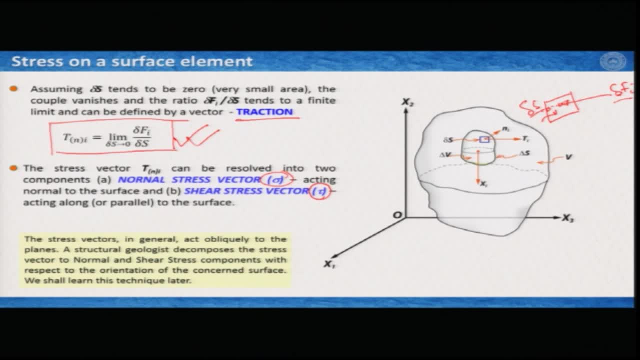 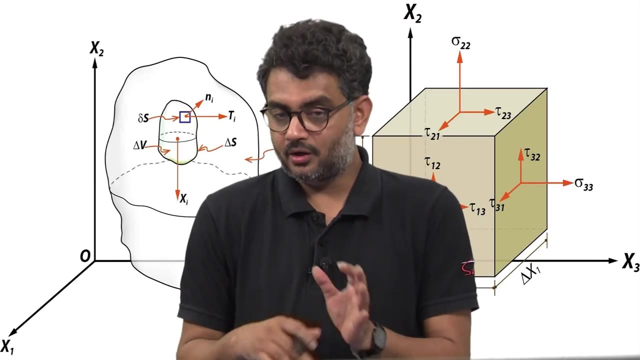 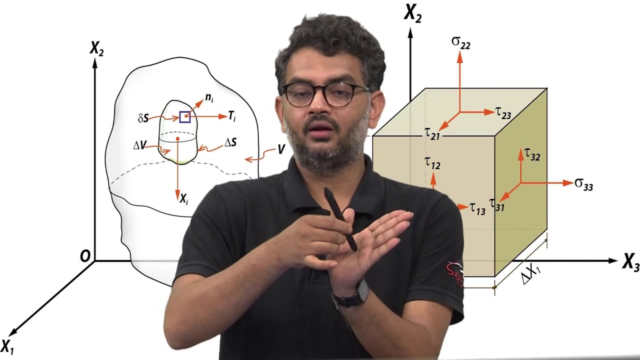 geologist therefore has to decompose the stress vector to normal and shear stress components with respect to the orientation of the concerned surface. Now, we will learn about this technique later, but what I try to convey with this statement- that if we have a force acting on this surface, we can immediately resolve it to the normal. 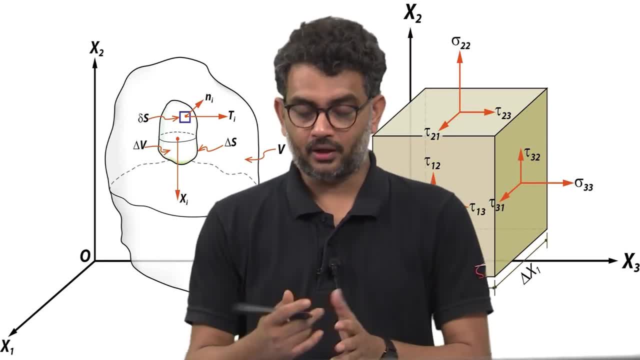 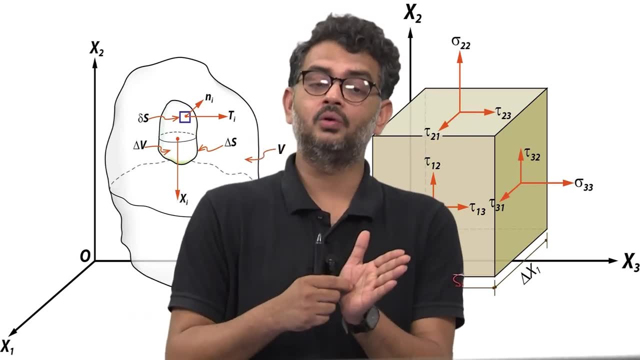 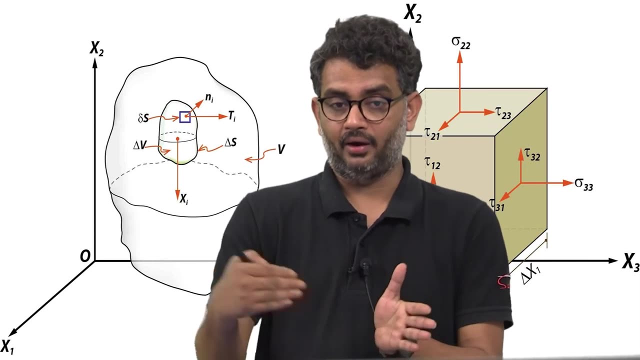 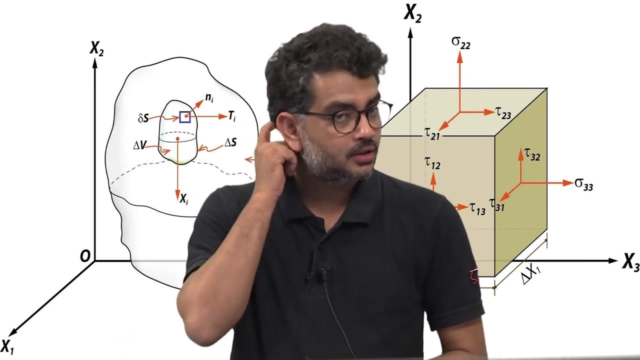 and stress component by simple vectors. But for stress or for traction it is not that straight forward because you have to also consider the orientation, the area and its orientation where the traction is working with. Now, once we have more or less a steady idea that what is stress, at a point now we would 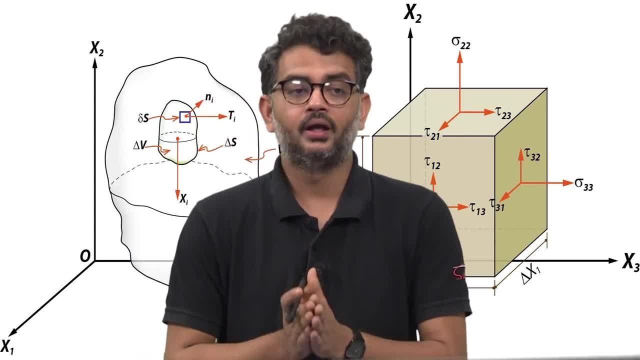 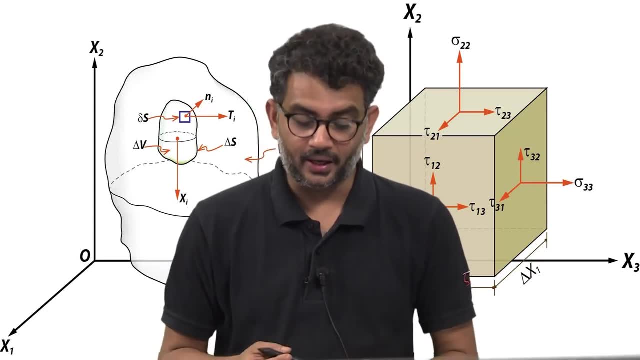 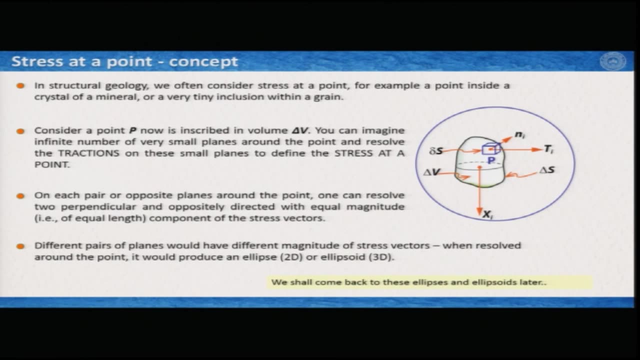 like to see stress on a surface, and then we would like to switch to another part, and which is even more relevant, that is, stress at a point. So let us talk first about the concept. as I said, in structural geology we often consider stress at a point, For example, a point inside. 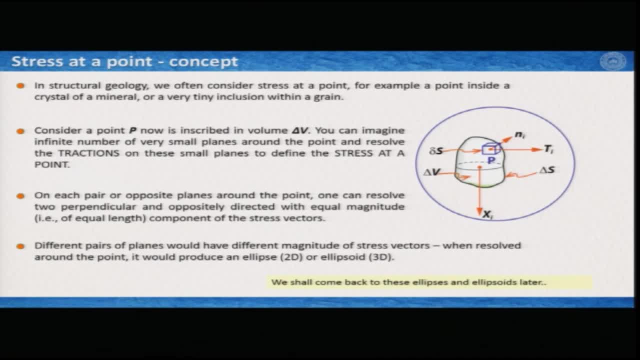 a crystal or mineral or a very tiny inclusion within a grain, and we would like to know what is the stress acting, or what is the stresses in this point. Now we will follow the same process. So we have the same drawing. again, we have this. 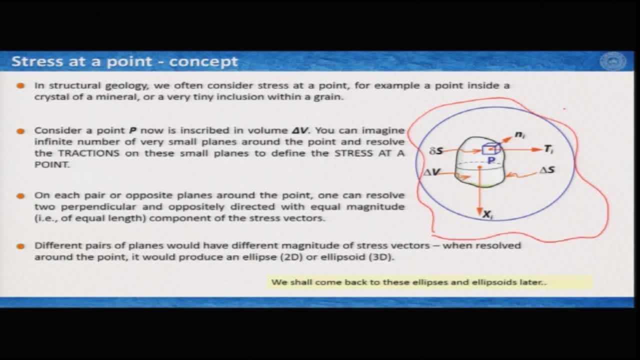 volume V somewhere out- And I just highlighted the area here where you have del V- then you have delta V, delta S and then del S- small surface, And we have again the same point P, along which or on which we have already derived. we have generated a very small surface and we looked at how. 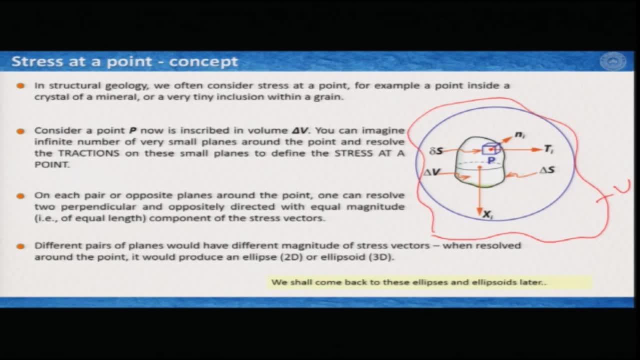 we can get the stress on a surface resolved. So the stress at this particular point, if we consider a point is now inscribed in the volume del V and if I consider this as a point P, then it is possible. actually I can draw. 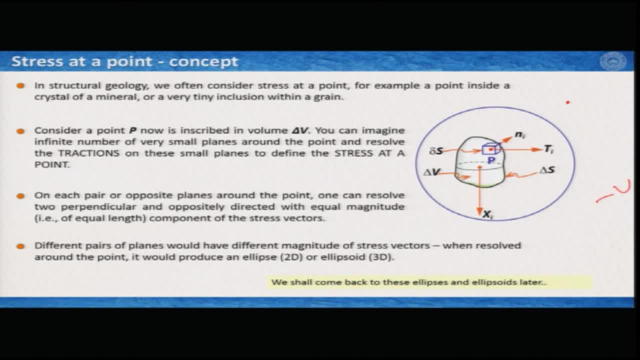 infinite number of surfaces around it. What I mean by this? if I have this point P, then I can draw infinite number of surfaces, and so on. Now, these surfaces are very small because these are around a point And on each surface. 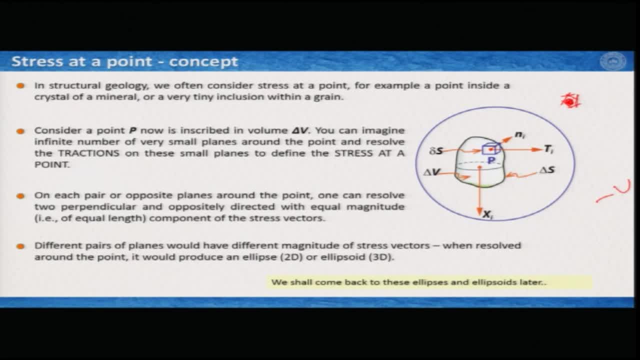 we can calculate what is the stress because stress, classically is defined as reactive force per unit area. So, in short, that you can imagine an infinite number of very small planes around the point and resolve the tractions on these small planes and define the stress. 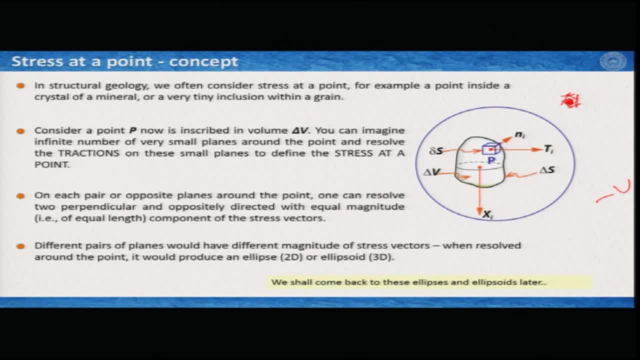 at a point. Now this is some sort of approximation or consideration, And these areas have to be very, very small. Now, on each pair of opposite planes around the point, we can resolve two perpendicular and oppositely directed with equal magnitude, therefore equal length component. 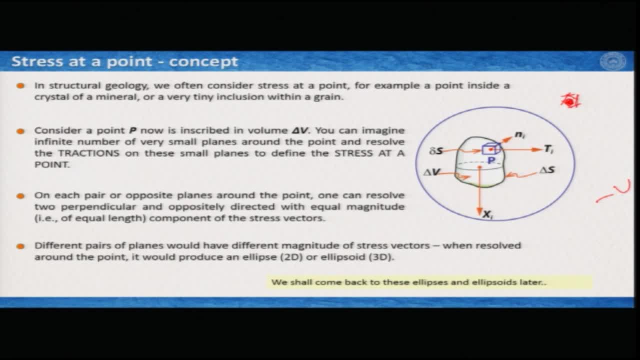 of the stress vectors. We we will learn about it very soon, If I have a little point here. and I have two planes oppositely directed, I have two planes oppositely directed, I have two planes oppositely directed, and so on, and a force is acting. 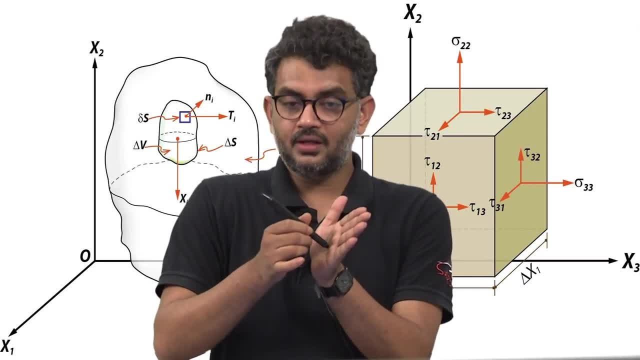 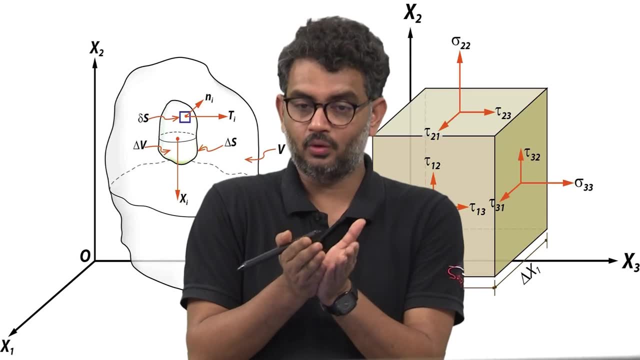 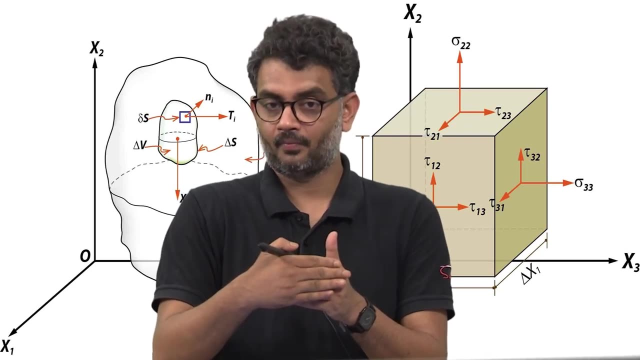 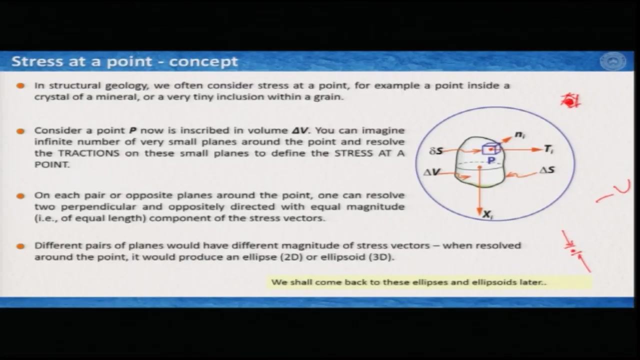 on this plane, then it is highly possible that this oppositely directed magnitudes are equal, but with other pair of oppositely directed planes the magnitude may be different. That means, if I have a point here, I have two surfaces. it may be acting like this and I have two. 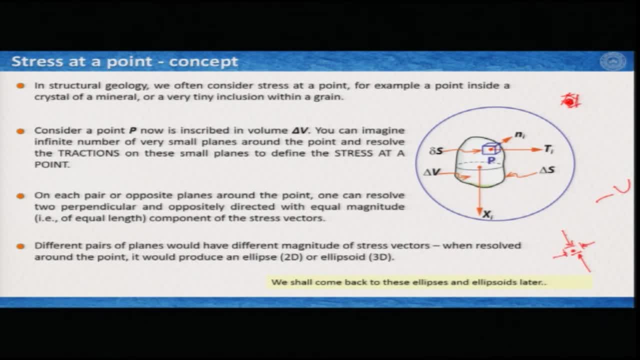 points here, the magnitude in these two cases. here and here the magnitudes are same but their magnitudes are different in the other two pairs. So if I consider many such planes and these magnitudes may vary constantly, and this would come or this would finally yield: 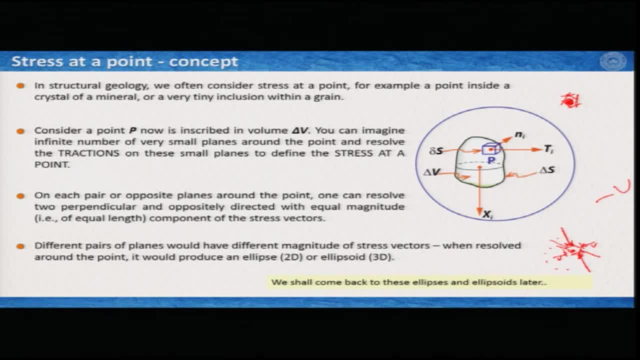 what we would call very soon as stress ellipse when you consider it at 2D and what we would call stress ellipsoid when you consider in three dimension. But before that, let us again come back to this particular topic: stress at a point. Now what we can do. 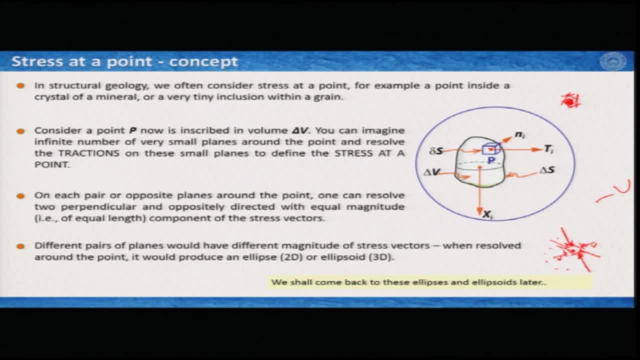 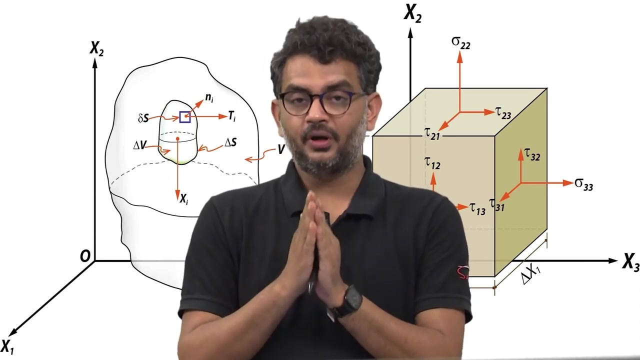 Actually, we can draw a very small unit cube around this point P, considering six of these many surfaces that is possible to draw around this little point. Now, these six surfaces, one pair of each, are aligned, perpendicular to one of the principal axis of stresses. 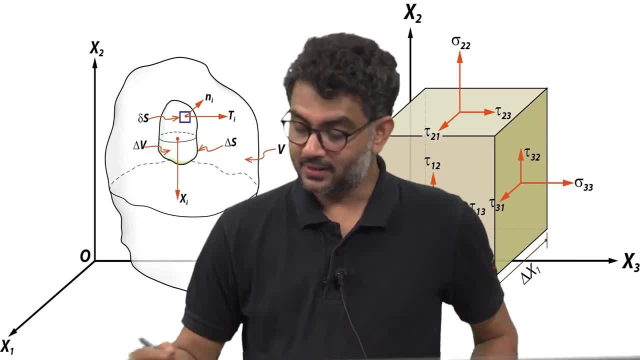 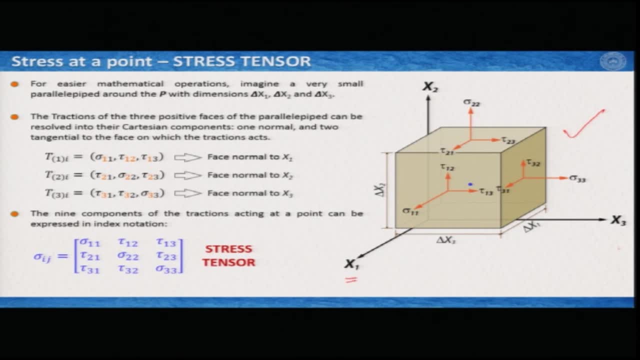 So how it would look like. It would look like something like this: what we are seeing here. We have these reference frames in Cartesian coordinates: x 1,, x 2,- sorry, x 2- and here is x 3.. This blue dot here. 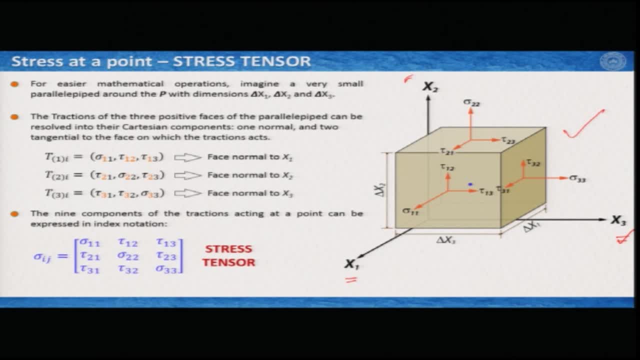 is the point P, and we have considered six planes. in the positive side we are seeing now three planes. there are, of course, the three planes on the other side. So this plane where I am marking, So this little dot, is perpendicular to your x 3,. this plane is perpendicular to your x. 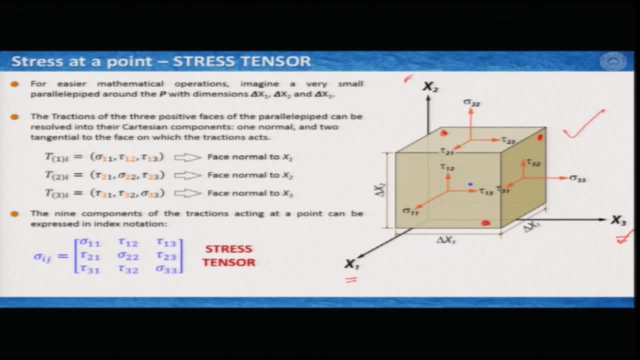 2 and this plane is perpendicular to your x, and these three planes and their opposite planes hold this point P, So this is a very magnified view of around a point P. Now we know that a force is acting. Now we know that a force is acting at a point. 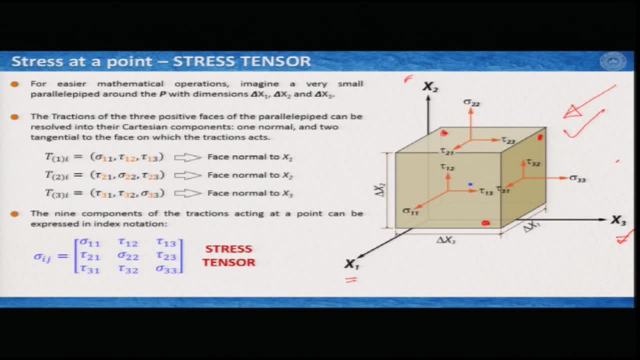 P and it is acting here And for each surface we have defined, following a traction, that there should be a normal stress and there should be a shear stress. Now, normal stress for the normal stress. if we consider this plane, which is perpendicular to the x 1,, the 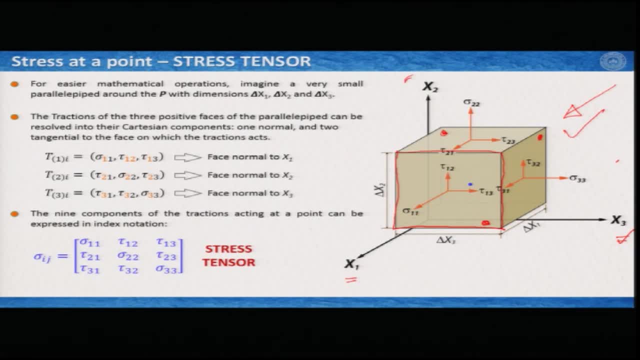 normal stress on this plane, which is perpendicular to X1, certainly would be directed along the X1 direction, which in this case is sigma 11.. Now the shear stress. again, we can resolve it in two different components, because one would go along the X2 direction and one would go towards the X3 direction. 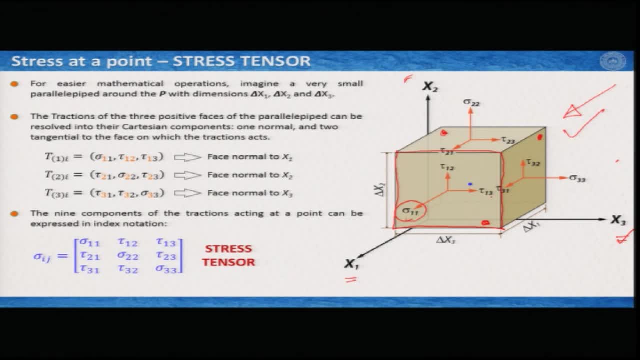 So we actually get three mutually perpendicular set of stress components, one of them which is a normal stress component, and two of them are the shear stress components, and one of these two is aligned to X2 and this one is aligned to X3.. And a similar case happens if we consider the plane which is perpendicular to M irgendwie. 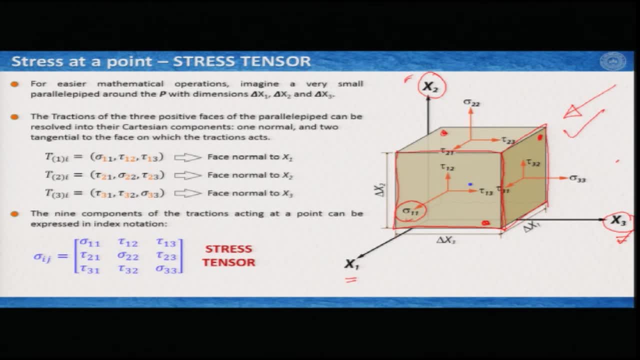 V unfold 잦. so perpendicular to X3, that means sigma 33 is a normal stress component, working along the direction of sigma 33, then two shear stress component, tau 32 and then tau 31.. And then, similarly, on this plane which is perpendicular to X2 direction, we would have normal stress. 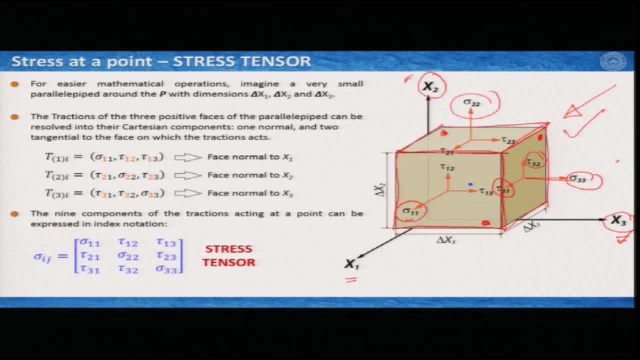 component which is acting towards X2, and then two shear stress components. Now you have seen that three different nomenclatures or different notations are given. Let me explain what it is What we see on this plane. I come back again to this plane. So, sigma 11 tau. 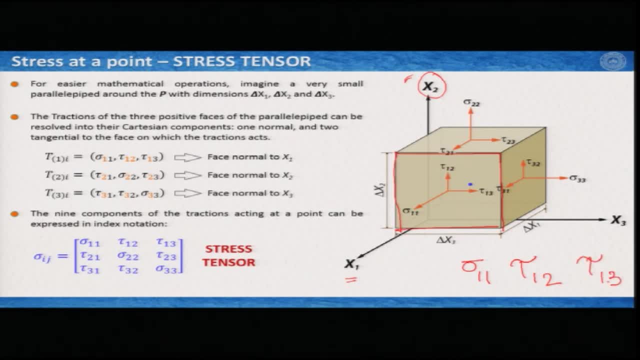 12 and tau 13.. In this case, this first index in each of these stress components indicate the plane it is acting or the plane perpendicularly it is acting. So in this case this plane is perpendicular to X1.. So therefore, in all cases this is first component. 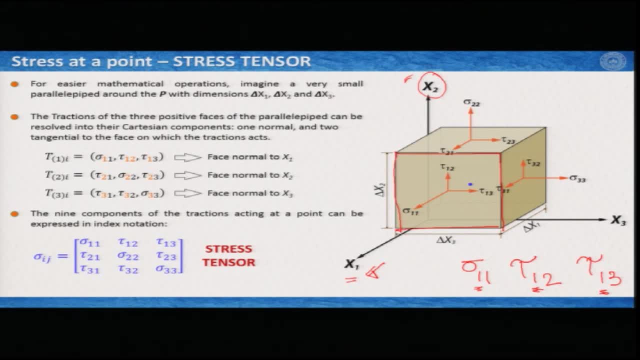 is acting. That means this sigma, this tau and this tau. these stresses are working on a plane which is perpendicular to X1 direction. The second component, 1,, 2 and 3, are the direction along which the stresses are working. So in this case, the second component here is 1.. So it 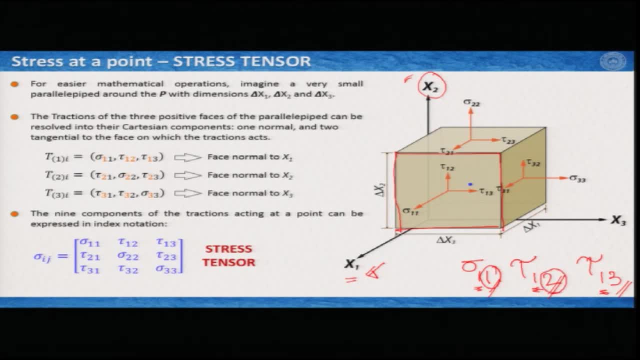 is working along the X1 direction, Then 2, second component is 2.. So this is working along the X2 direction, and this is 3 tau 13.. 3 is the last component, So it is working along the X3 direction, And this is: 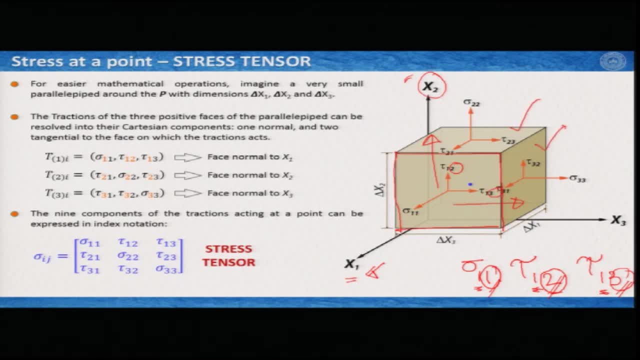 also obvious or applicable for the other two planes, The other three negative planes that we do not see in this image and exactly oppositely directed, but similar magnitude stresses would, But similar magnitude stresses would work there. So if we now come back to our traction, 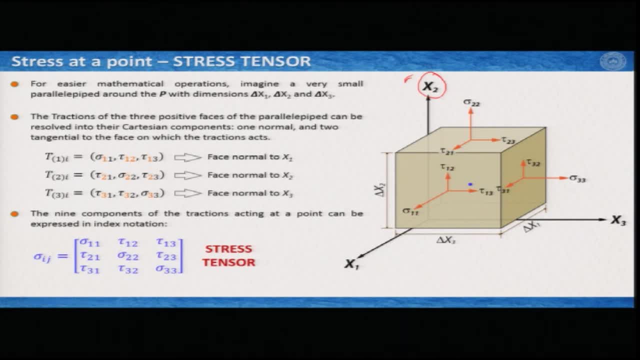 idea or what we have learnt from the traction. So on each surface we have, in this case this is parallel to, or, sorry, perpendicular to, X 1.. So here I can- I am sorry- here I can write that this is T 1, that means traction working on the plane, which is perpendicular. 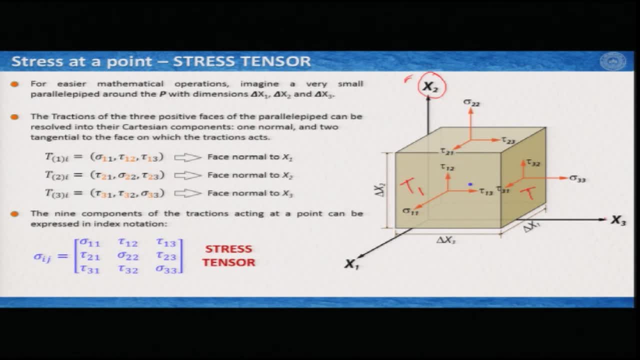 to X 1, traction working to perpendicular to X 3, which is T 3, and this one is T 2.. Now, for each of this- T 1, T 2 and T 3, we see that we have three components to define. 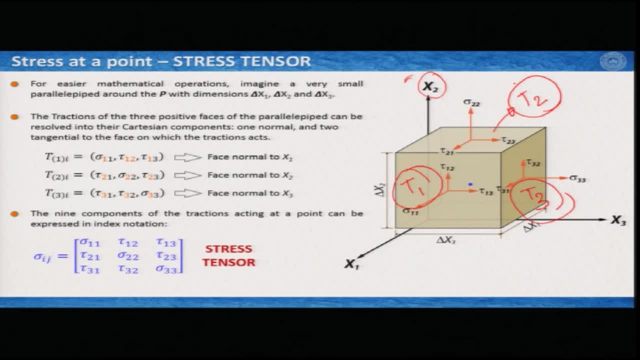 the stress on this plane which is perpendicular to X, 2. But everything we are doing to define the stress on this plane which is perpendicular to X, 2. But everything we are doing to define the stress along this point P, So to define the state of stress along this point P, we 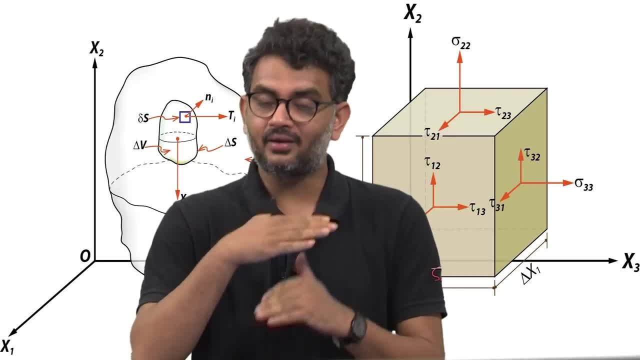 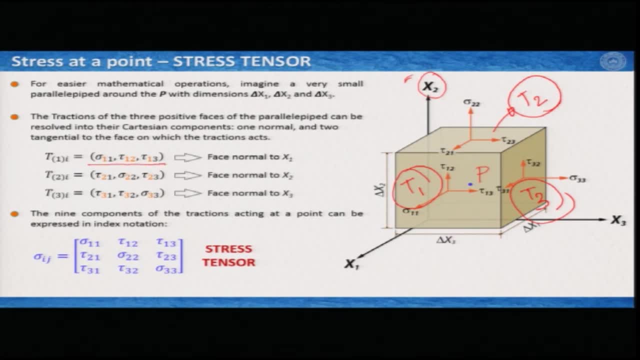 first have to resolve the stresses acting along the three surfaces. So for T 1, we see that this is sigma 1: 1, tau 1, 2 and tau 1, 3 for the face normal to X: 1, tau 2, 1, tau. 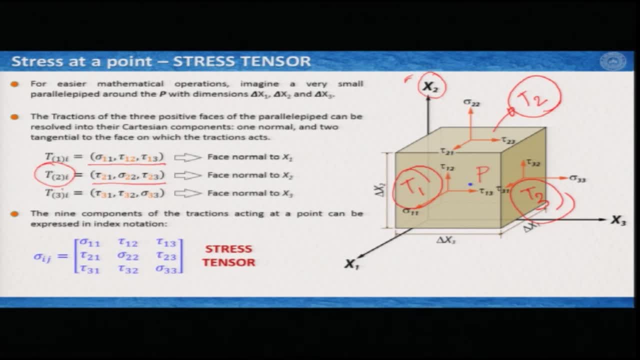 2. For a traction two and then traction three is tau 3, 1, tau. I am sorry, this must be tau 3: 1, tau 3: 2 and sigma 3: 3, which is normal to X 3.. Now all these nine components. 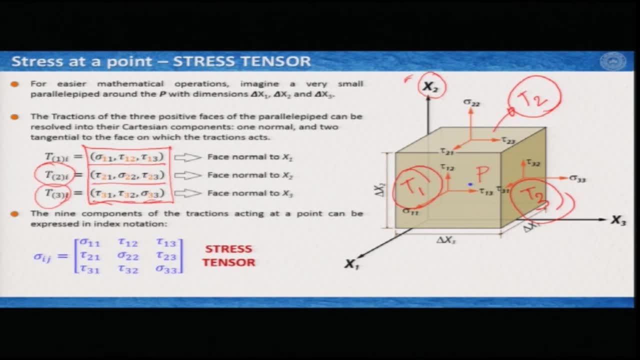 that we see here are required to define the stress at this point P And each example of Each of them. as we have understood this: T 1, T 2 and T 3- these are tractions and tractions are vector. but when we need all these nine components- 1, 2, 3, 4, 5, 6,, 7,, 8,, 9 components- 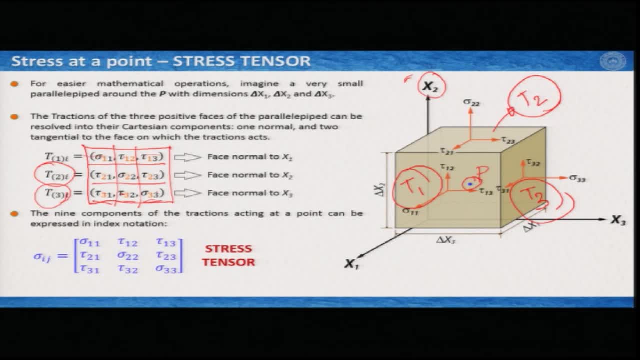 to define the stress. at a point it does not remain a vector anymore. It comes to a new component or new sort of dimensions or description of the parameters, and this is known as tensor. So you can write these three components in a matrix form: sigma 1- 1,. tau 1- 2,. tau 1- 3,. 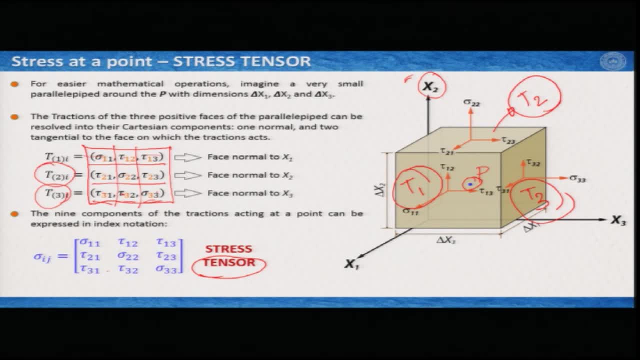 tau 2 1, sigma 2 2, tau 2: 3, tau 3 1, tau 3: 2 and sigma 3: 3, and you can simply notify or note it in the form of index notation: Sigma i, j- and this is your stress tensor, which is neither a scalar quantity nor a vector. 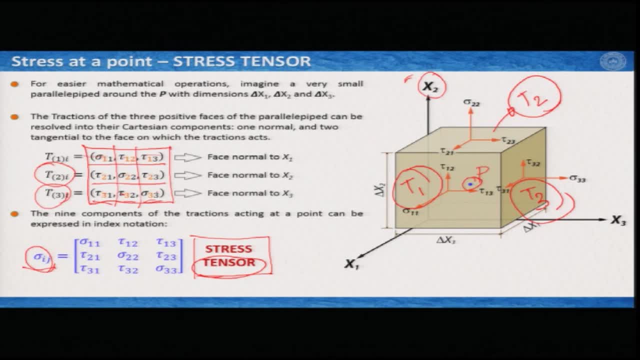 quantity, but a tensor, and I tell you this is a second rank tensor. So force attraction was a first order tensor and stress at a point is a second order tensor and this is neither a vector nor a scalar. Only, if you have now the idea that from the traction, which was a vector, now we arrive. 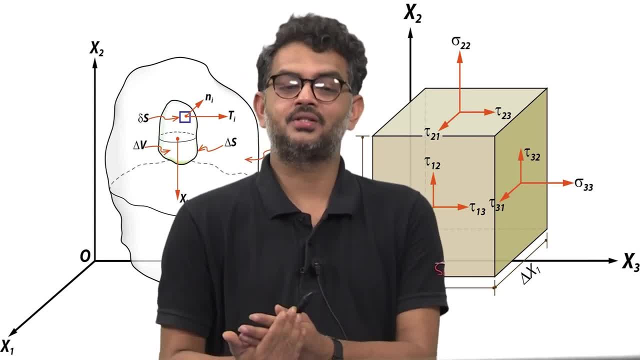 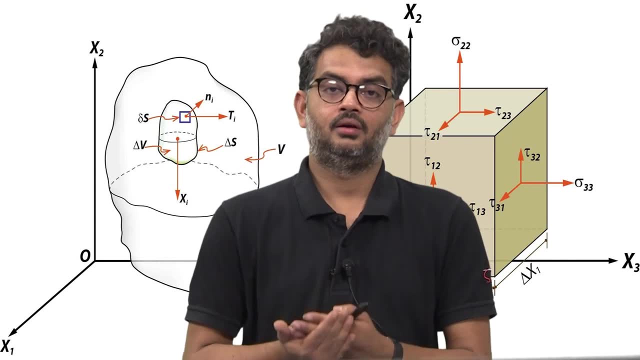 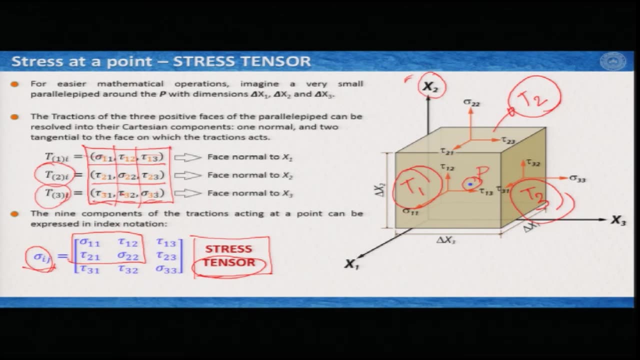 to a new concept when we have to define the stress at a point we can. it cannot be a vector, it is a tensor, and in three dimension you need nine components, and in two dimension you can define it only with four components, but it would still remain a tensor. Now there. 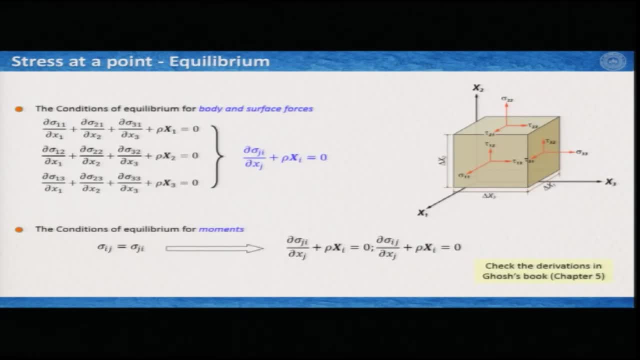 are some fundamental equations that we need to, that we need to know or learn, and which is known as equilibrium concepts of stress tensor. I am not deriving this equations but, as I have noted here, you can get this from the book- one of the books I referred- Professor SK Ghosh's book, If you go to chapter. 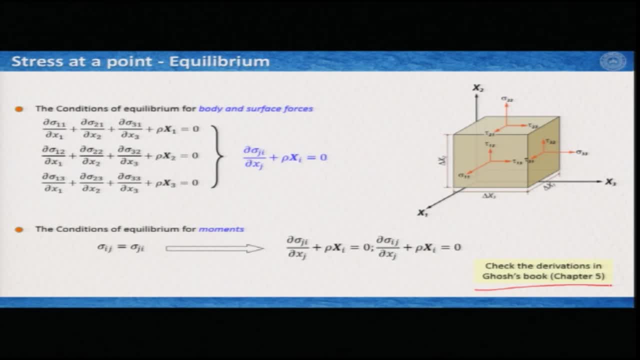 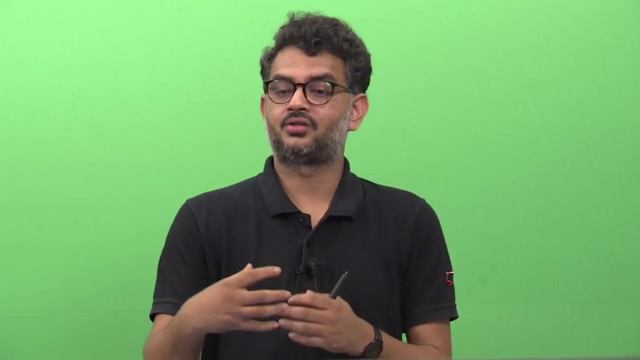 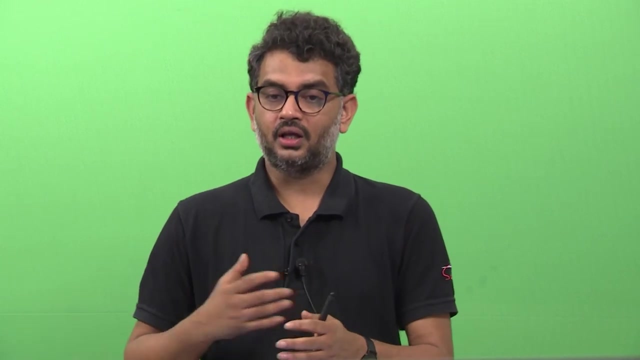 5,. we can see what is this. but the concept of this equilibrium, or stress equilibrium, is that this cube would stay in a static mode. That means it does not translate along x 1,, x 2 or x 3 direction, or it does not rotate. So if it has to translate, then we have to. 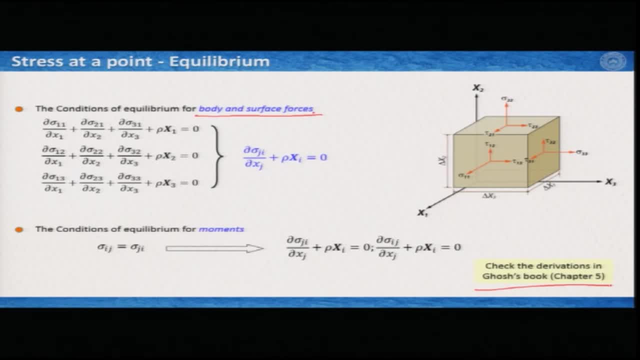 consider the body and surface forces. That means body and surface forces. the sum of body and surface forces in a particular direction should be 0. That means they are balanced. So this is for x 1 direction. this is for x 2 direction. this is for x 3 direction. 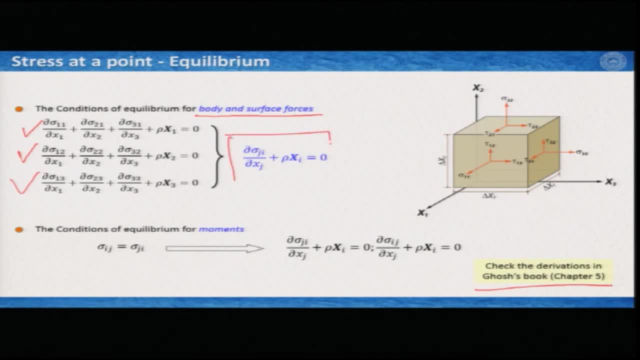 You can get these equations and in index notation form you can write it this way: And if this is not rotating, that means it is not rotating this way, say, for example, clockwise. Therefore, this tau 3: 2 has to be 0. 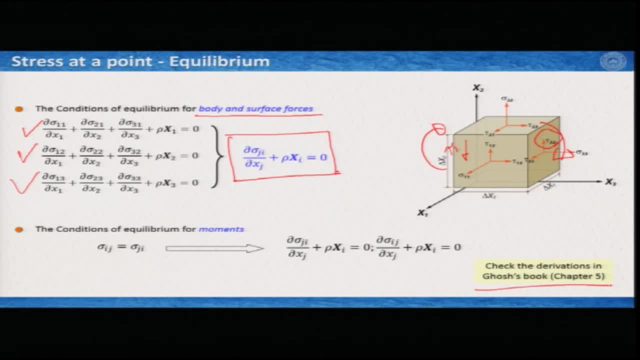 It has to be counter balanced by, on the other side, tau 2, 3.. And we can show that in equilibrium condition this is possible. That is the only condition that it does not rotate. So this is the equilibrium that we consider for moments And therefore it defines, as I said, tau 3. 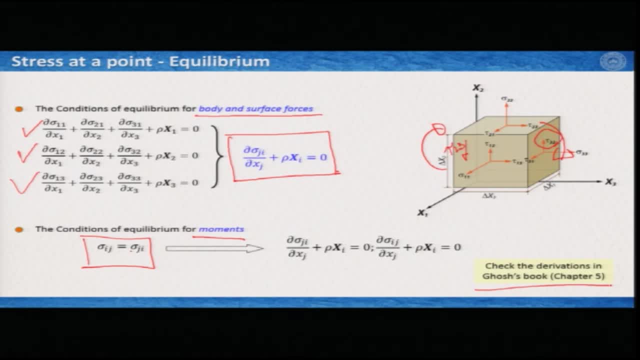 2 has to be equal to tau 2: 3.. Therefore, sigma i j should be equal to sigma j i. when your body is in equilibrium, And therefore here we had sigma j i, You can simply represent sigma j i to sigma i. 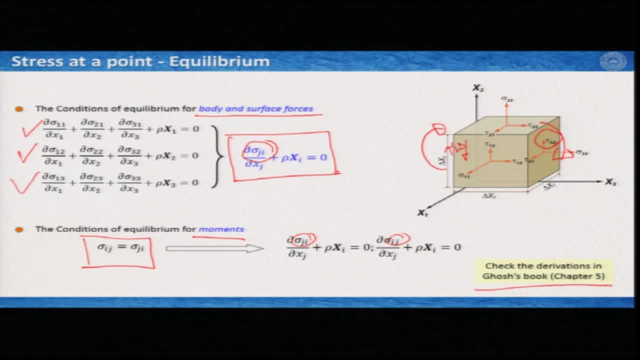 j. I did not dedicate too much time on this because you can get these derivations from other books, But I hope you have now understood the concept of stress on a surface, which is a vector- traction And stress- at a point. 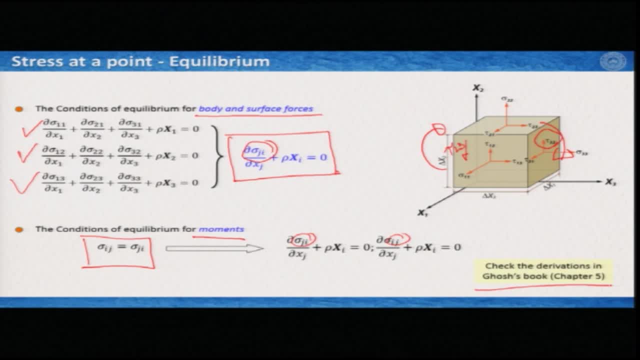 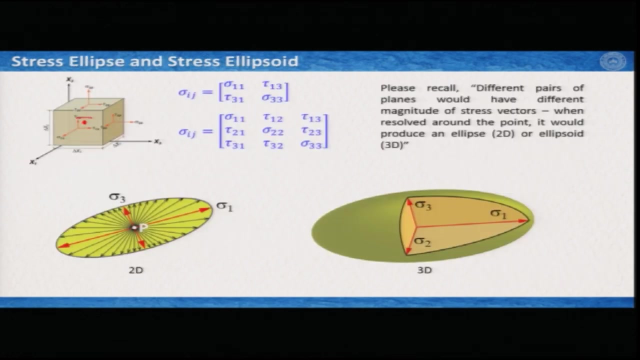 Now let us come back to the concept of stress ellipse and stress ellipsoid. As I said that on this particular point P here we can consider n number of planes surrounding this point P And oppositely oriented planes would have same magnitude. that means same length, but different directions, different senses of. 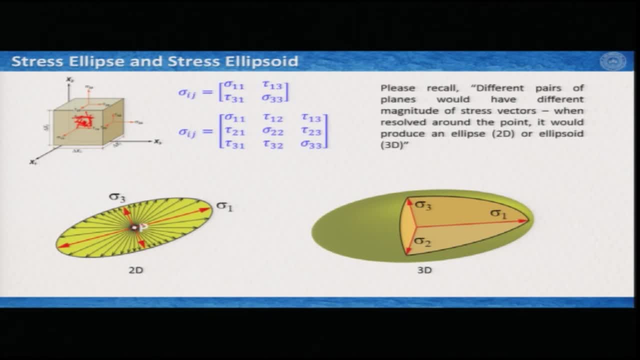 action. So if we look at- this is the point P here- And if we look at in two dimension, then we may get actually. So these are actually, for example, if I consider these two red arrows. So around these we had this plane and this plane around the small arrows, small red arrow. 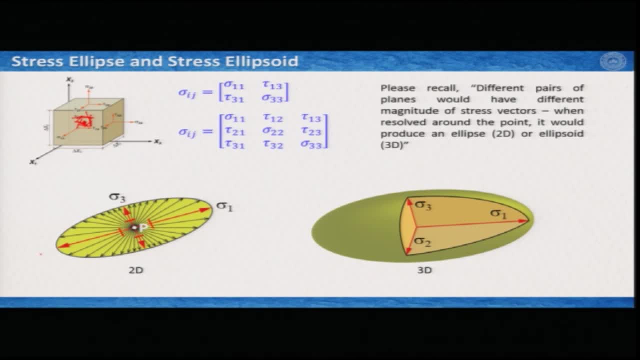 we had this plane, So here it is working on this side, here it is working in this side. Their lengths are equal, that means magnitudes are equal, but their orientations or action directions are different, and similarly here. Now, of course, you can have n number of planes. 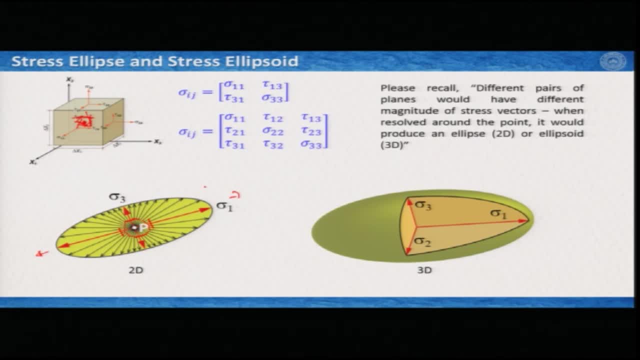 around it And you can draw their normal components with their respective magnitudes. So if you connect all these points, you certainly would get or end up with these points. So these are the kind of points that you can have, And this ellipse is known as stress ellipse, when you consider in two dimension, The maximum. 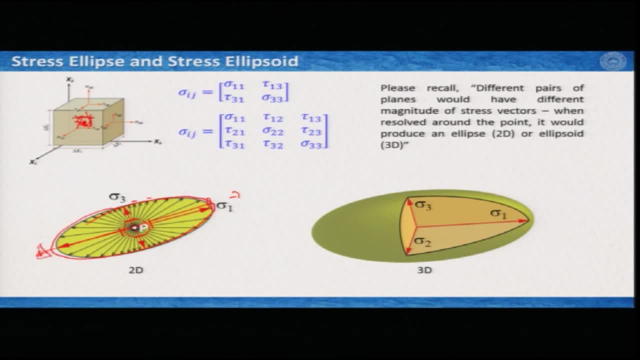 length you get will define it as sigma 1.. And the minimum length you get of this stress magnitude will define it as sigma 3.. In three dimension, very similar to the strain ellipsoids. we look at it get a very similar shape. 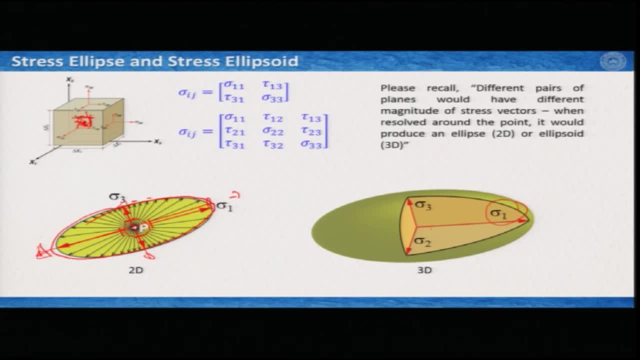 maximum we would get sigma 1, at the minimum we get sigma 3 and intermediate we get sigma 2.. Now, what is sigma 1, sigma 2 and sigma 3, and how does it differ from this sigma 11? 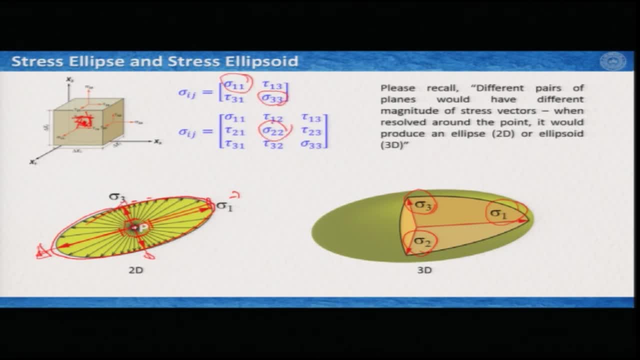 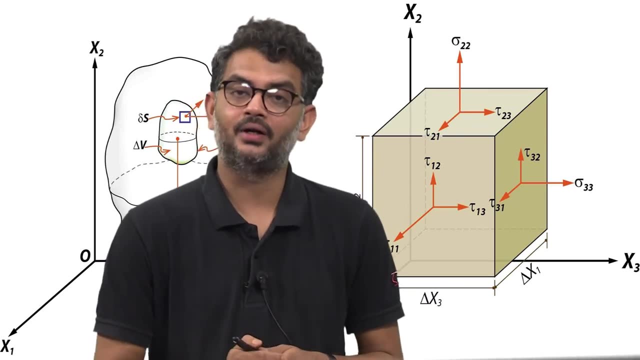 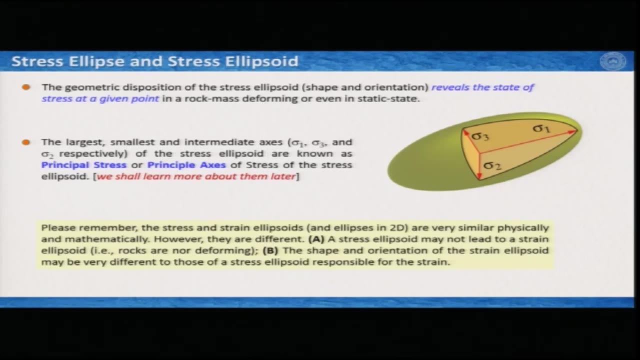 or sigma 33 or sigma 22,. we will hear it in the next lecture, we will learn it on this next lecture, but before that let us get some more ideas about the stress ellipsoid. So the geometric disposition of the stress ellipsoid, its shape and orientation, is generally described. 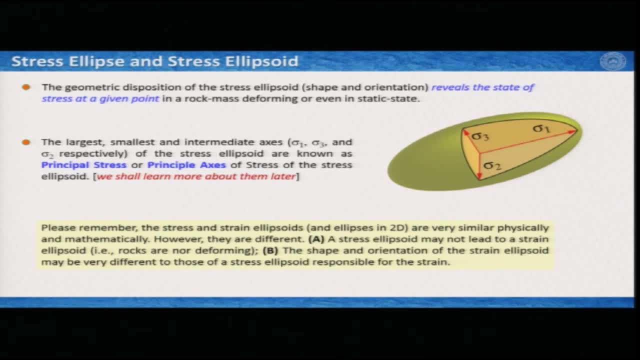 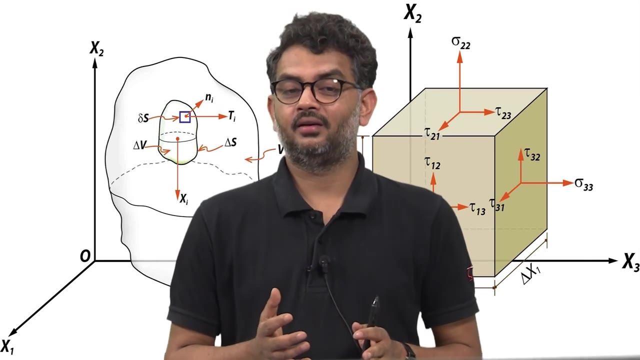 by the stress ellipsoid and it reveals the state of the stress at a given point in a rock mass deforming or if it is even in a static mode. Now, this is something very important that we have just learned. not necessarily you have to deform a material that there is. 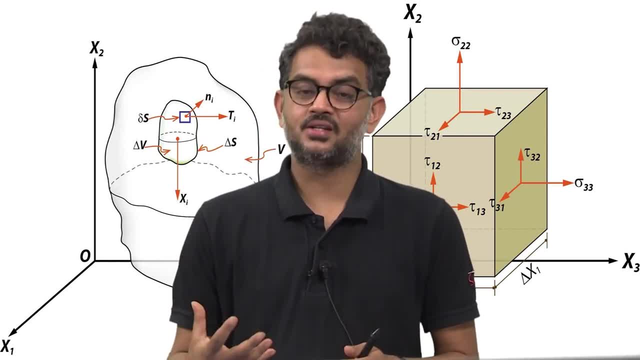 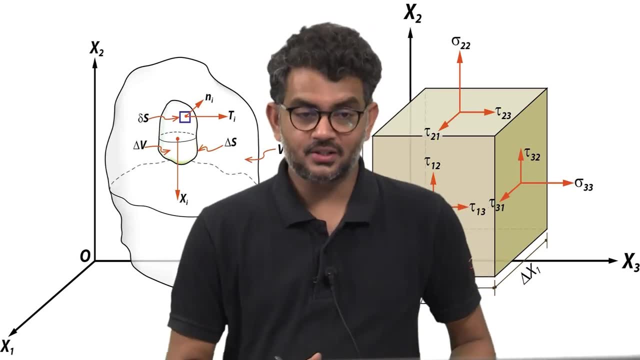 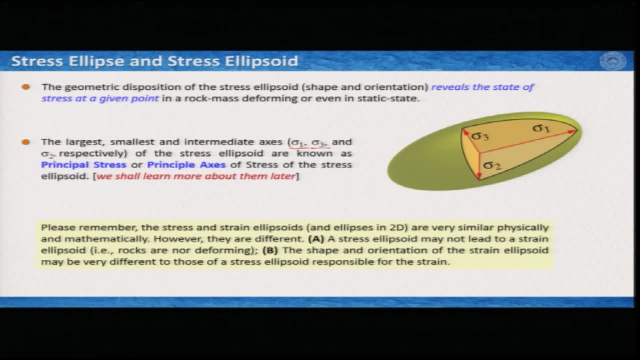 a stress or because there is a stress, not necessarily the rock mass has to deform. and we have just learned that the largest, smallest and intermediate axis, which will define sigma 1, sigma 3 and sigma 2 respectively, of the stress, ellipsoids. 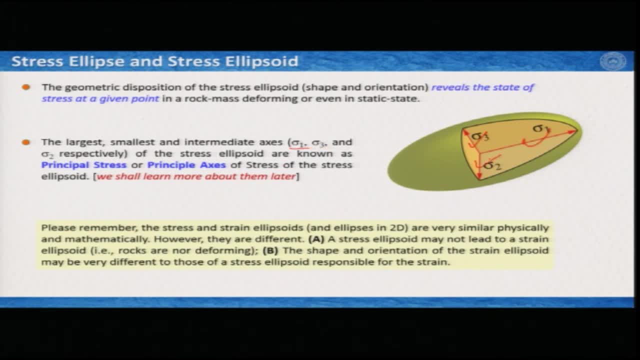 Stress. this one, this one and this one are known as principal stress or principal axis of stresses of the stress ellipsoid. This is something which is very interesting. will again learn about it later in the next lecture- but let us have some very basic ideas that 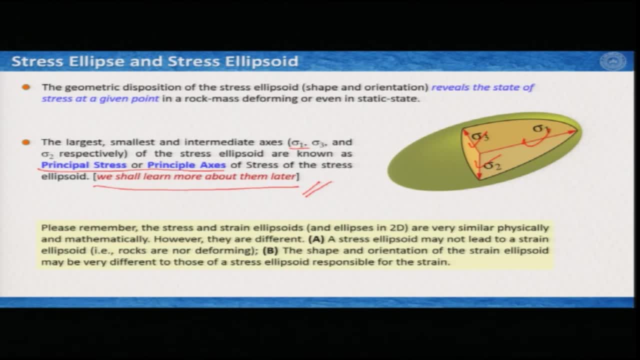 the stress and strain ellipsoids. they look very similar. I just change the colors but But they look very similar. their physical appearances are very similar. their mathematical descriptions are also very similar. However, always remember that these are different. A stress ellipsoid may not lead to a strain ellipsoid- that I just said that rocks are. 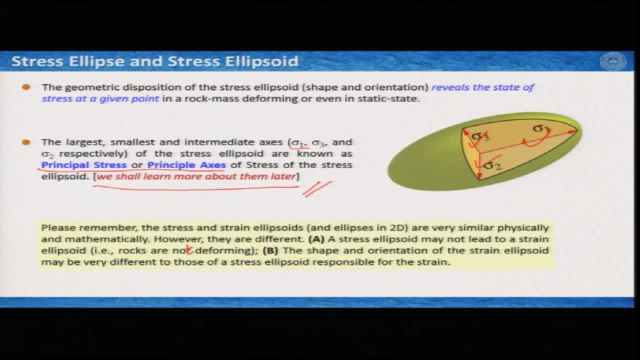 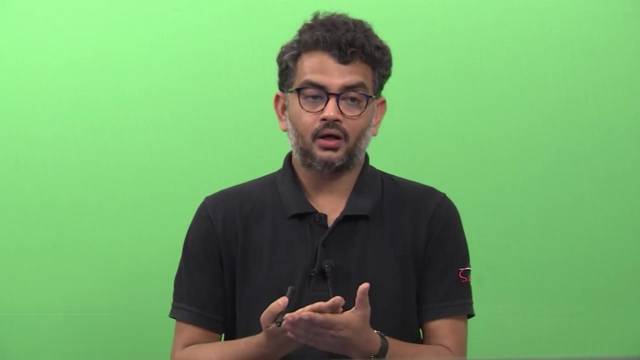 not deforming And, importantly, the shape and the orientation of the strain ellipsoid may be very different to those of a stress ellipsoid responsible for the strain. And now we would see that what are compressive stresses, tensile stresses, shear stresses? 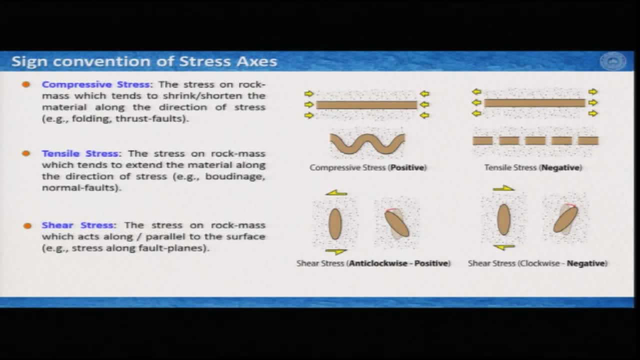 and what are their sign conventions? Now, compressive stress is the stress on rock mass which tend to shrink or shorten the material along the direction of applications, And if you have a domain of compressive stress, You form structures like folds, buckle folds or thrust folds. So, for example, if I have 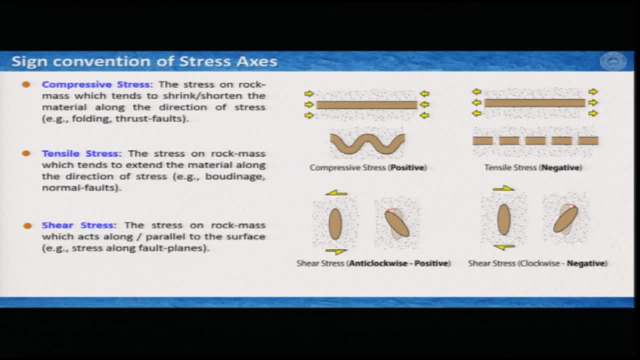 a layer embedded in a body, embedded in a matrix, and if I apply the stresses directing towards each other, I will produce a fold, and it is a compressive stress. If there is tension on the same layer, then I may produce a structure which we call buddhinas. we will learn about.